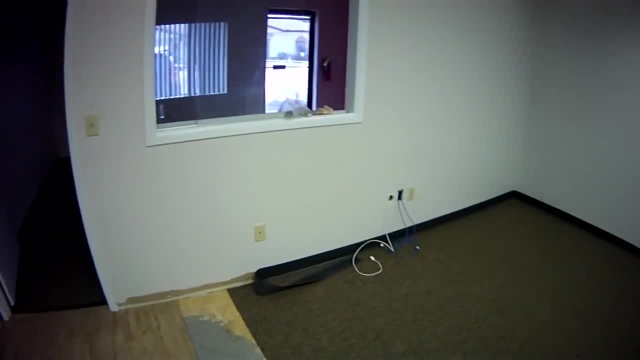 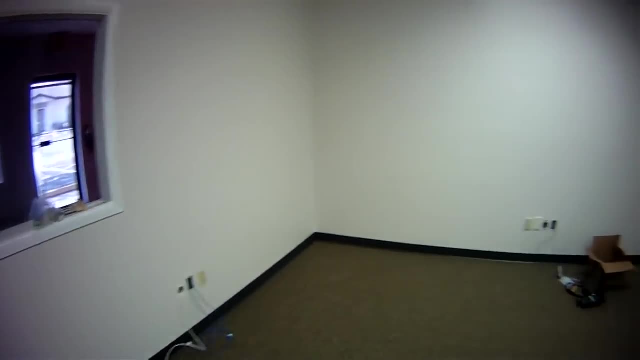 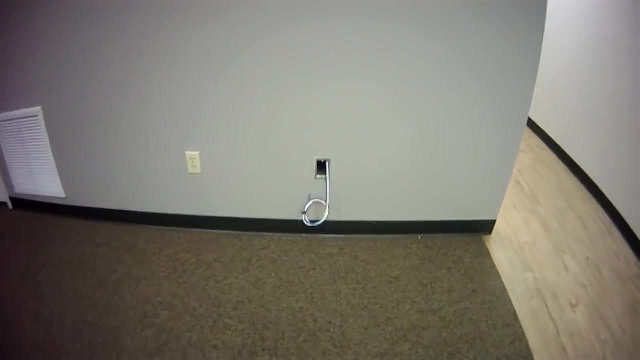 Hey there, this video is about installing network wiring in a small office, So I'm standing in what will become the reception area of a small doctor's office. You can see I've got three outlets that are in progress right now. One's there, got one over there. got one over there. 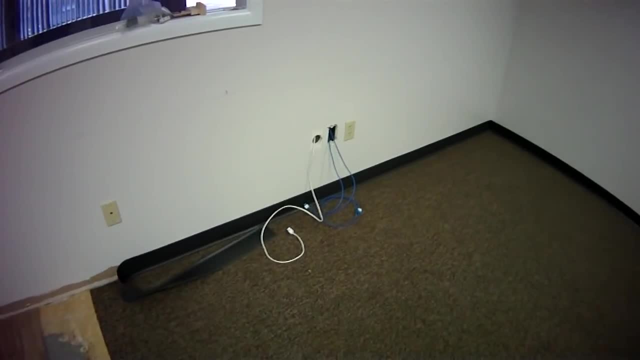 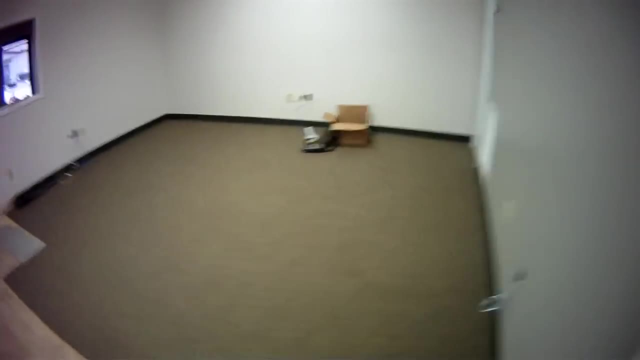 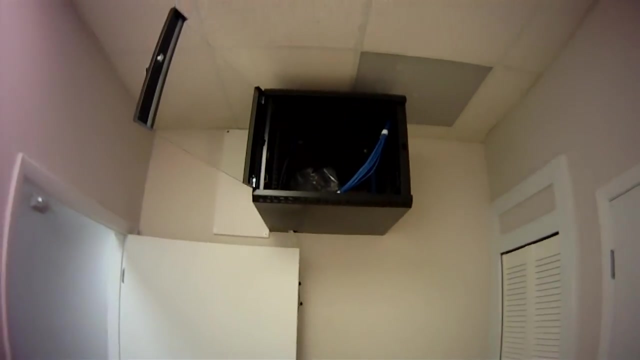 And the way that you wire up a network for a small office and actually, in a scalable sense, even for a big office. the idea is still the same. You start at one central location. So in this little room right here is our network cabinet. So this is our central location. 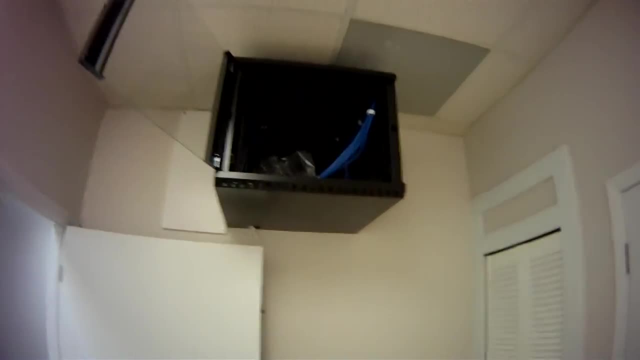 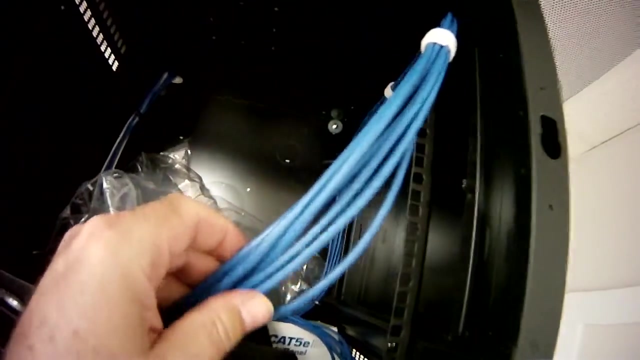 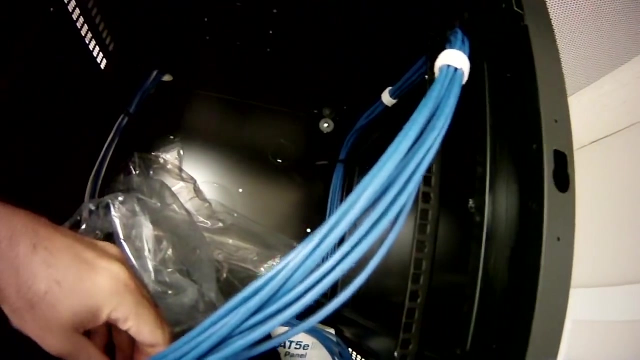 This is where all the network wires have to come back to, So this network cabinet has got the blue network cables inside of it. These are category five cables: Unshielded twisted pair cables that are for Ethernet, And you can get a box of that at. 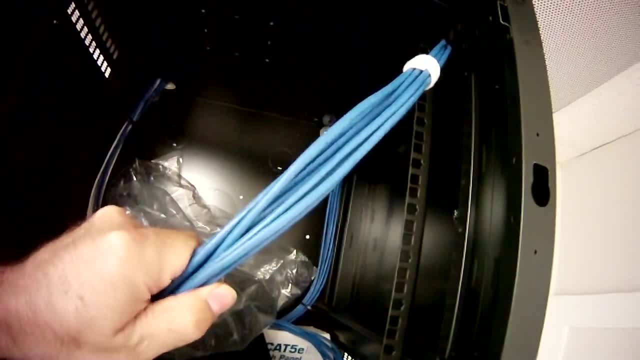 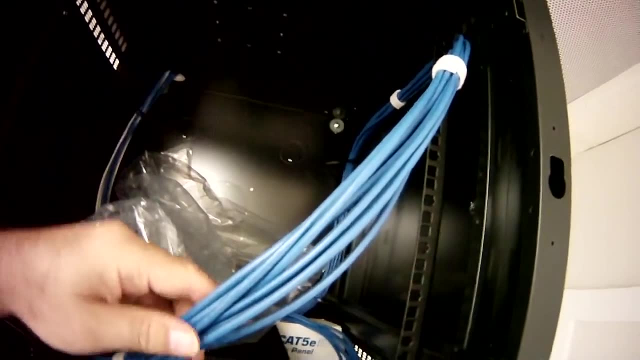 your local hardware store. Usually a box of a thousand feet cost about oh, maybe a hundred, maybe a little bit less. Fire rated's more expensive, so if you don't need fire rated, try to avoid that, Anyway. so what happened is I brought the cable box in here. that reel. 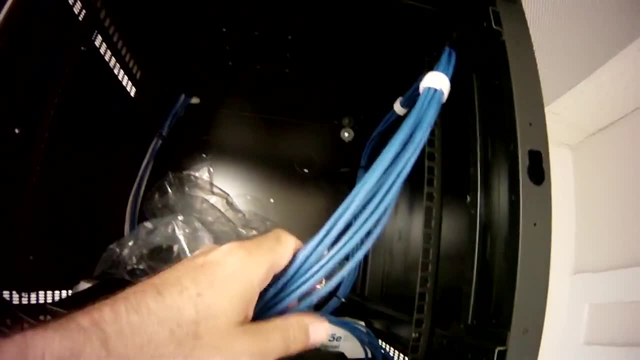 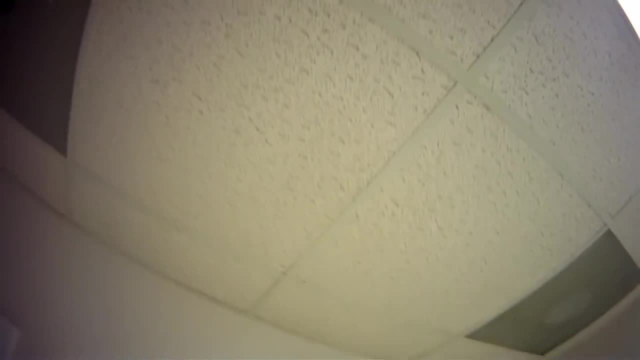 of a thousand feet of cable and I pulled these individual blue wires from this central point up through that hole, That hole back there into the ceiling. So you see this false ceiling here, these ceiling tiles, That's empty space up there. So if you've never had the opportunity to stick, 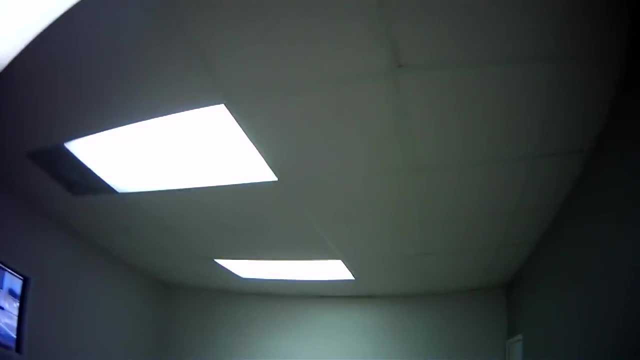 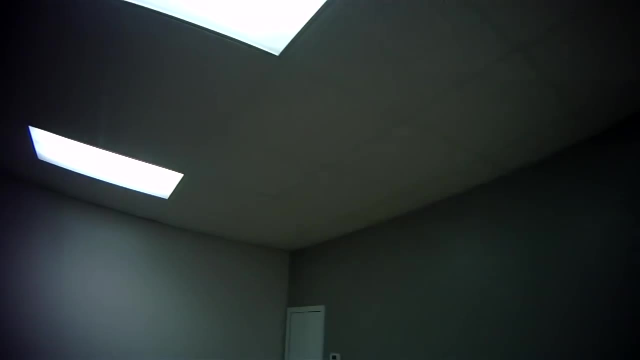 your head up there. usually there's just empty space above those tiles. Sometimes there's insulation on top of them, but generally you have anywhere from two to sometimes as much as six or eight feet of empty space up there. So you run those wires from that central point through the ceiling. So if you just imagine, 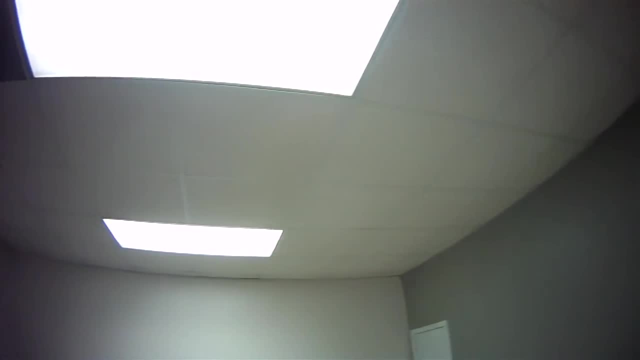 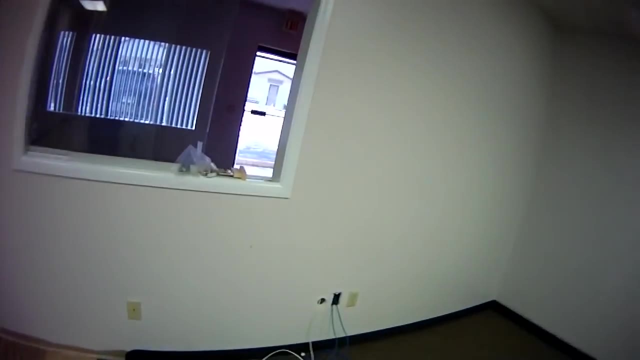 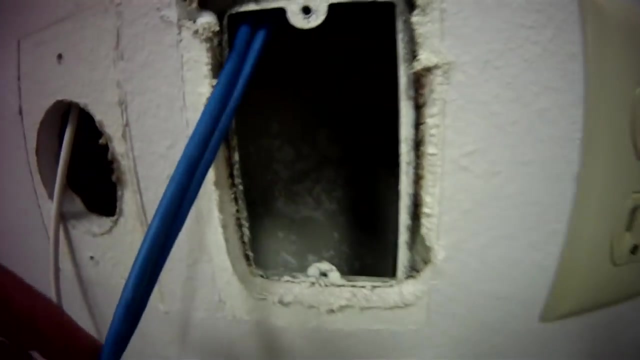 with a beemill if you will. if you could see up above those tiles, you'd see a couple blue wires going across the ceiling Above those tiles And then they come down the wall. Now, most walls in commercial construction are usually hollow, So if you can see, in there there's about three inches of empty space. 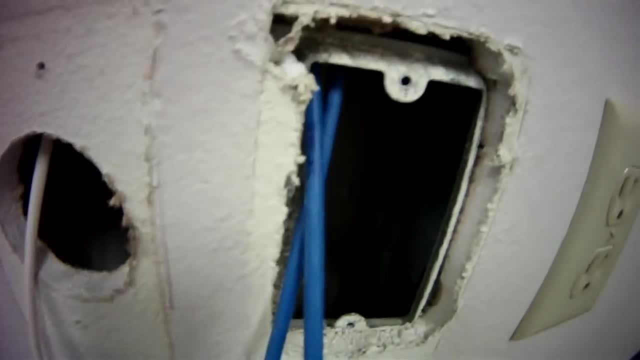 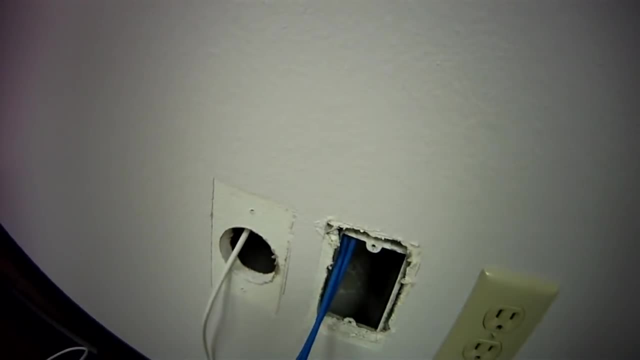 Sometimes they're not hollow, Sometimes they've got insulation in them, And then, depending on unique circumstances, you may have walls that just simply don't have any space at all, and that's a whole different ball of wax. But the short version of the story is you. 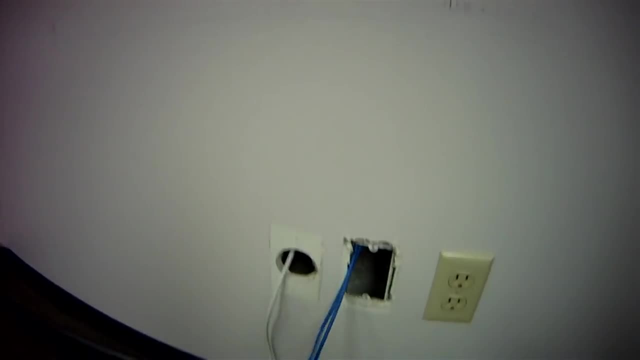 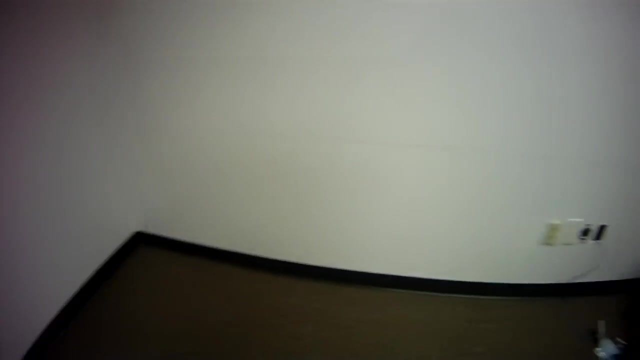 need to get these network wires from that central point where we just were to every outlet location where you're going to need an Ethernet connection. And then what you do is you put these Category 5 modular ends on them. Those modular ends then in turn fit. 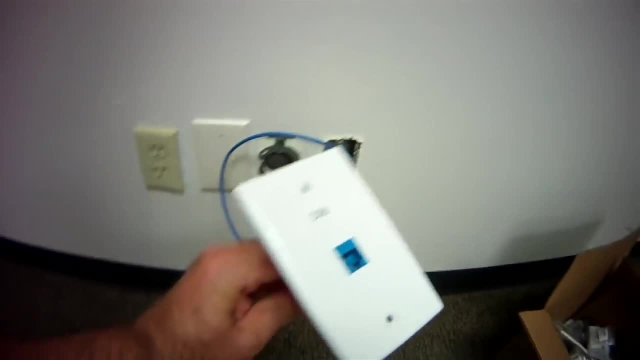 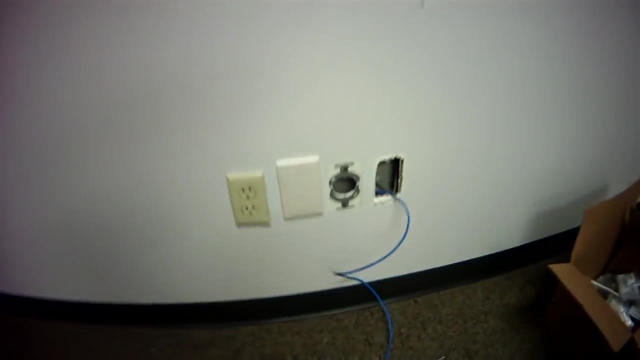 into a wall plate, And then the wall plate is labeled with a number. Now, why do we have to have a number? Well, the reason we have a number is so that we know that for that outlet right there, which is D06, which is short, 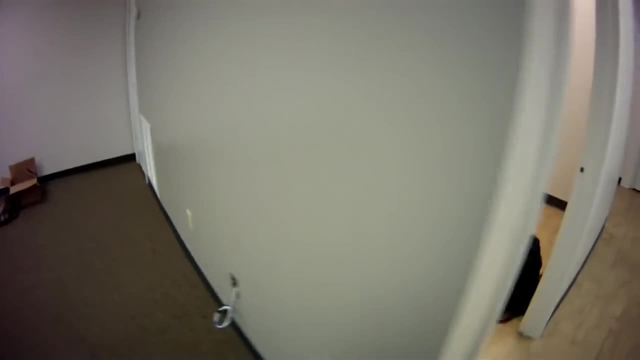 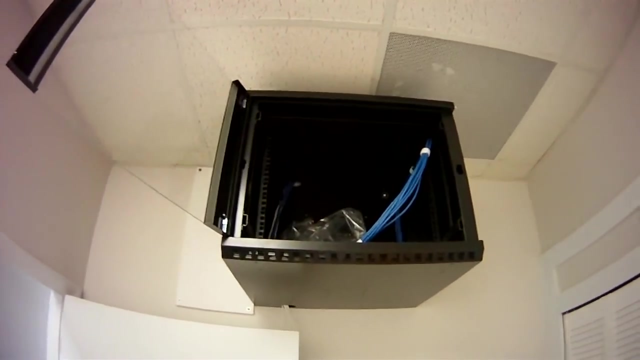 D06, which is short for data number six. We'll bring them back here and then I'll show you a little bit later. I'm going to mount a patch panel in here and that patch panel will have a one, two, three, four, five, six, et cetera, And that six will match the six. 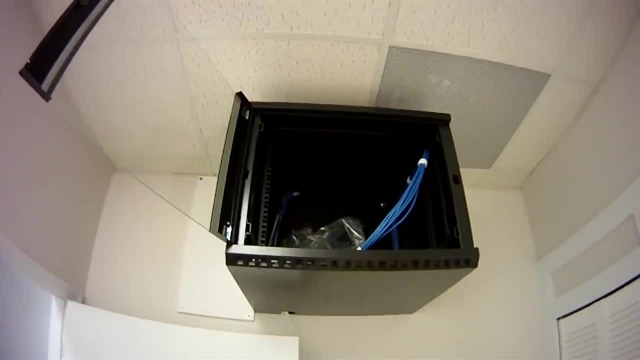 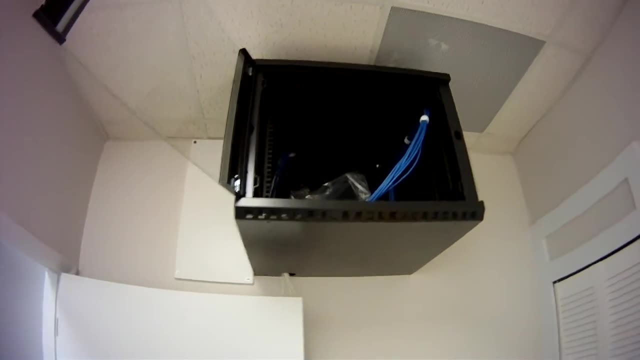 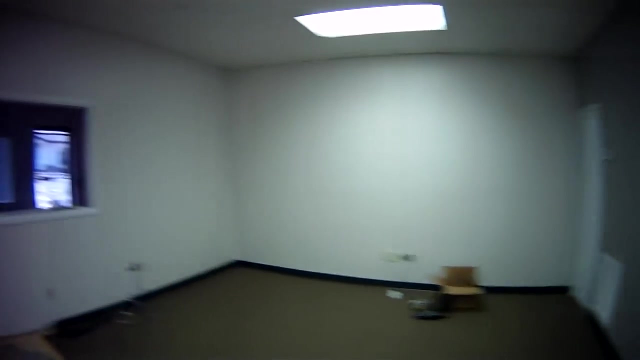 on the patch panel there. So that will become our horizontal network wiring system which we will use to connect the router or switches that will live in this cabinet out to all the various locations. So I've got a receptionist office. I've also got patient exam rooms. See, here's an outlet. 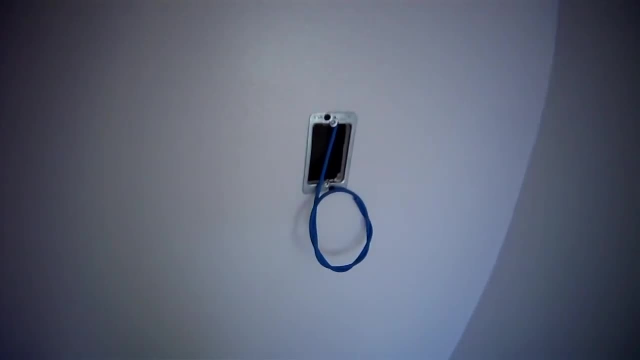 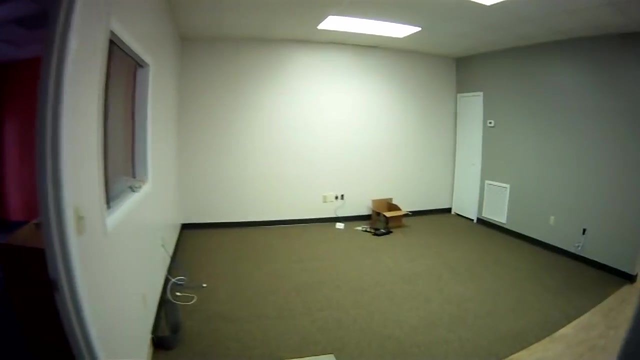 that I've run the cable to, but I haven't yet put the faceplate on yet. So when I'm all done, there'll be faceplates on all those outlet locations with a corresponding number that relates to the patch panel in the back, And then that will be my network wiring system. 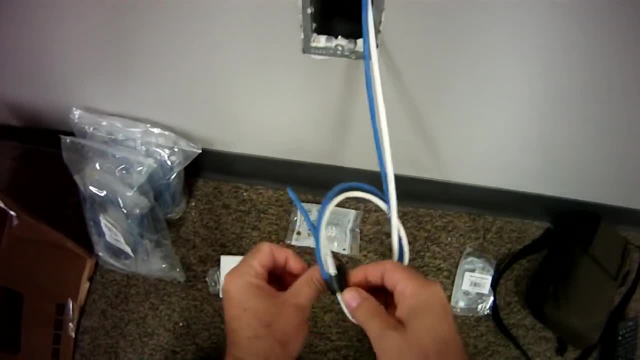 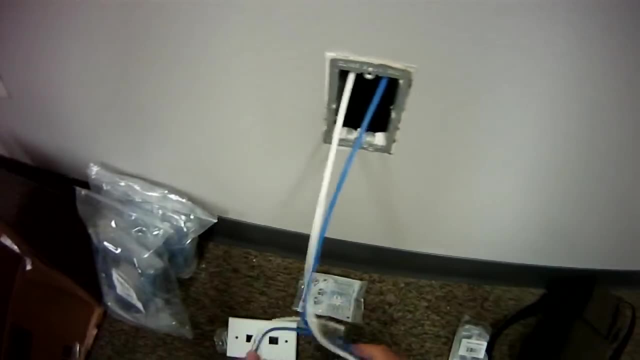 Okay, I'll show you a little bit more in a few minutes. Okay, So I'm going to do an outlet here for you, So I'm going to donate the. The slang word is RJ45.. The formal word is actually 8P8C. 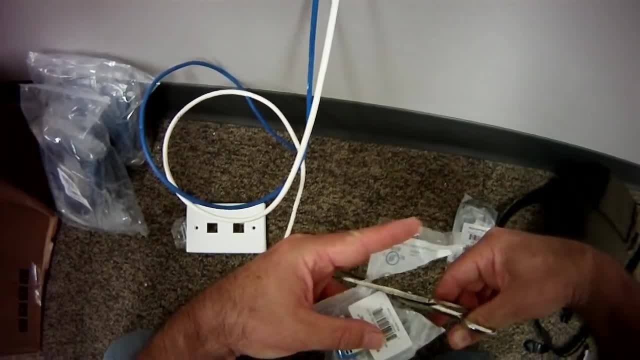 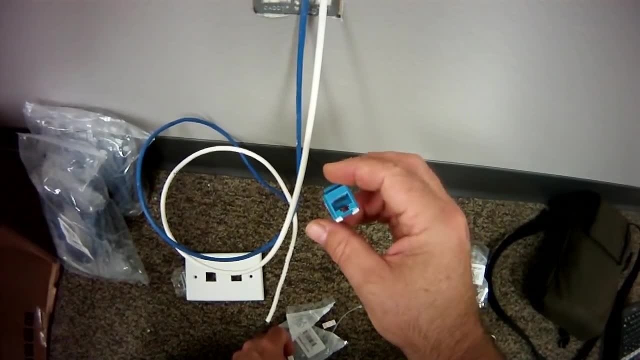 So, for instance, these little guys right here, these modular ends with the RJ45 end on them, They're called RJ45.. The real term is 8P8C, but 8RJ45 is what they get called a lot So. 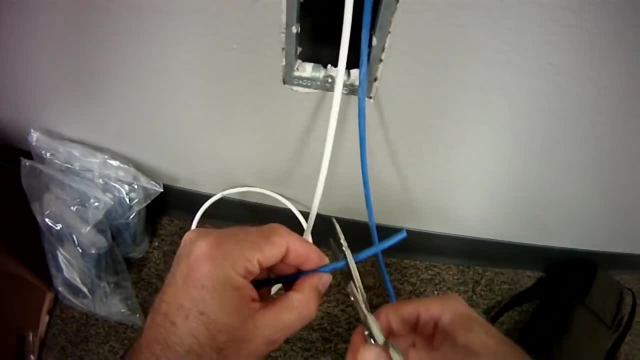 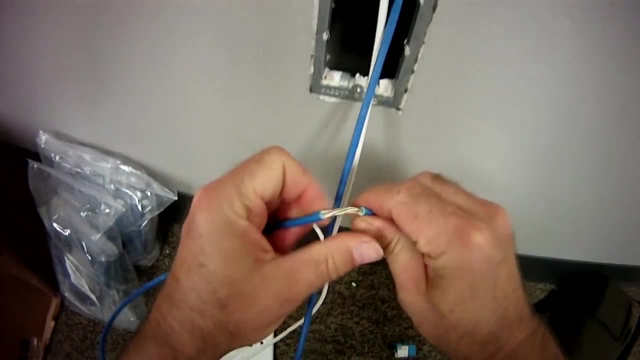 I've got this guy right here, Got my wire. I'll strip back some of the jacket. I kind of do this by rubbing my scissors on the edge and then some, Depending on the type of cable you work with, the cable might be brittle enough that you can just kind of snap it off and get rid of my excess rip cord. 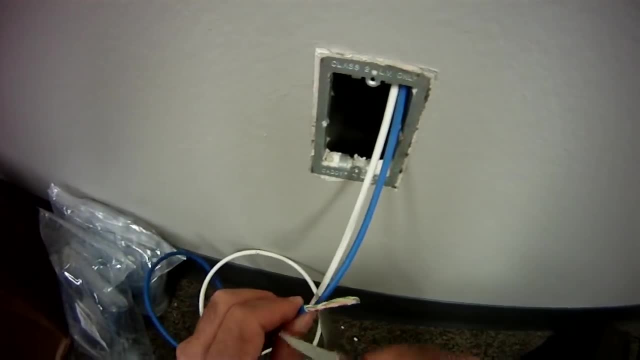 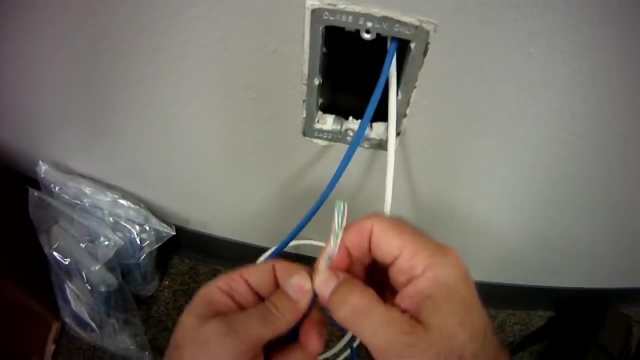 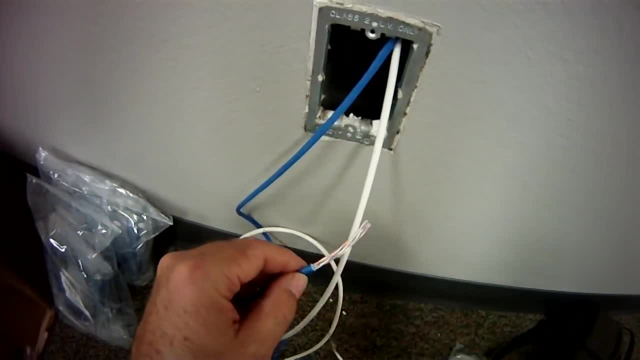 I've got a little bit of a. I've got a little bit of a. I've got a little bit of a. You know that opening cut like that with your scissors, But then take the rip cord and pull back some, like you're peeling a banana and get rid of the skin by cutting it off. 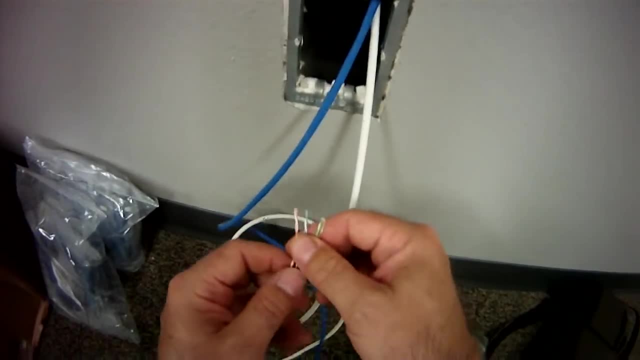 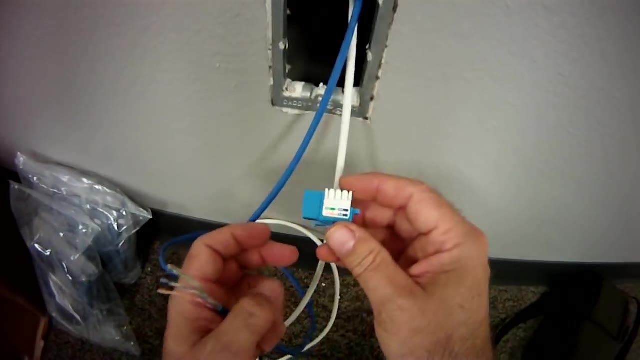 after that, because that way you avoid, you know, nicking the wires inside. Maybe when I do the next one, I'll show you that. Okay, so these jacks, depending on what brand you get, all come with a different punchdown. 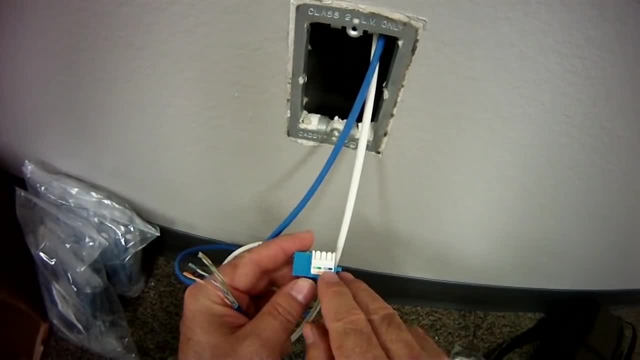 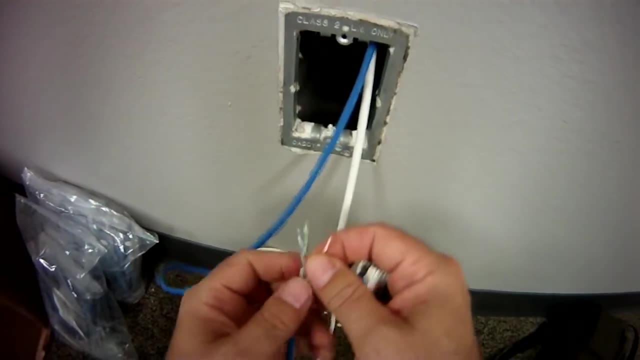 pattern, meaning see how this has got like a white, blue and then blue, then white, green and green, and you know white, orange and brown, white, brown and brown and so forth. They correspond to the colors on these wires. 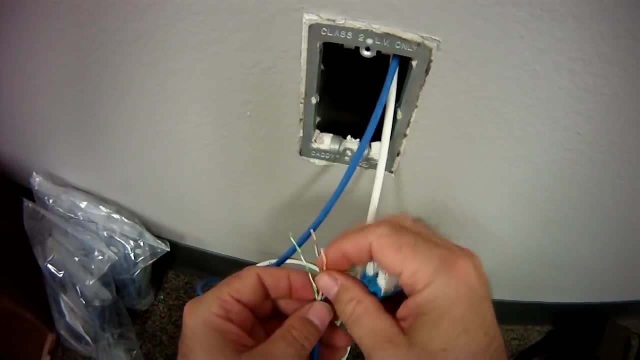 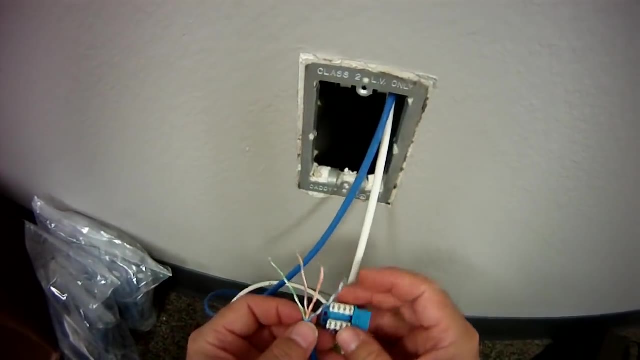 And you can look up other videos on YouTube about how to punch down a category 5 jack. So this is just kind of a quick and dirty to kind of help round out the video a little bit. But so what I do is I match the pattern of the wires. 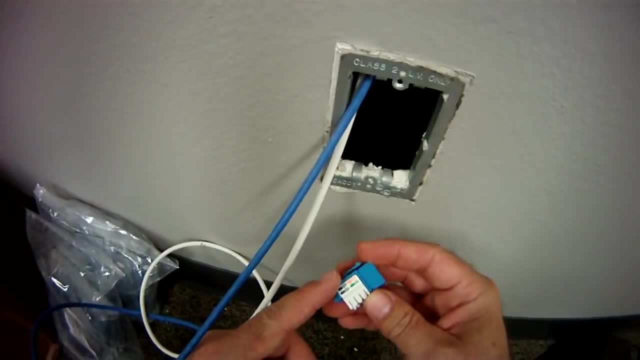 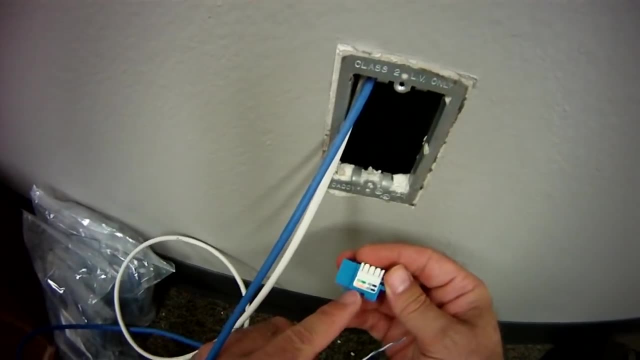 to the colors on the sides of the jack And, like I said, what I was going to say is that, depending on what brand of jack you get, this pattern could be different. So you have to just pay attention to the colors. There's two sets of colors here. 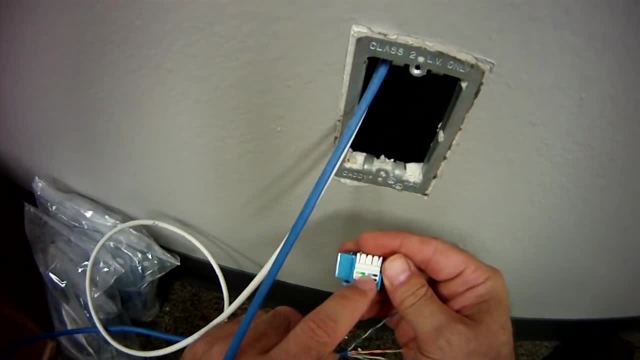 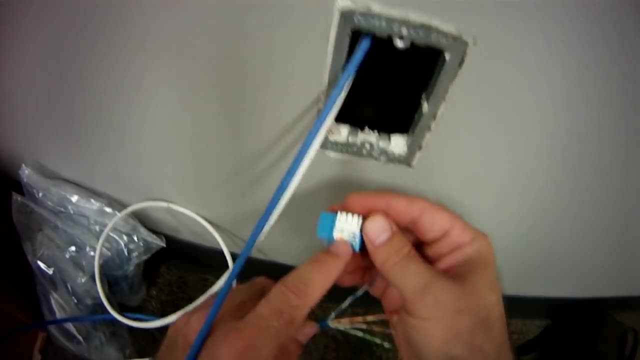 The top row is what they call 568A. There's a little bitty A right there, And the lower pattern is what they call 568B. There's a little B right there in the middle. So I'm going to be using B. B is the more commonly used wiring scheme. 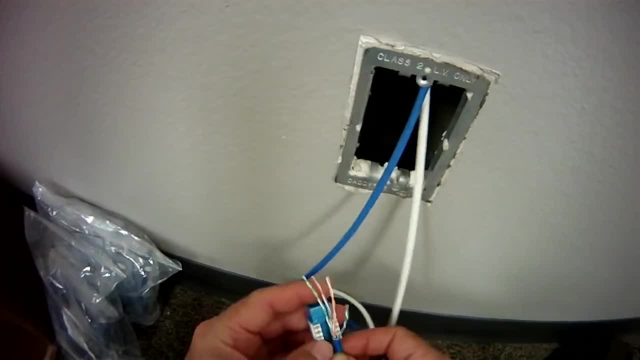 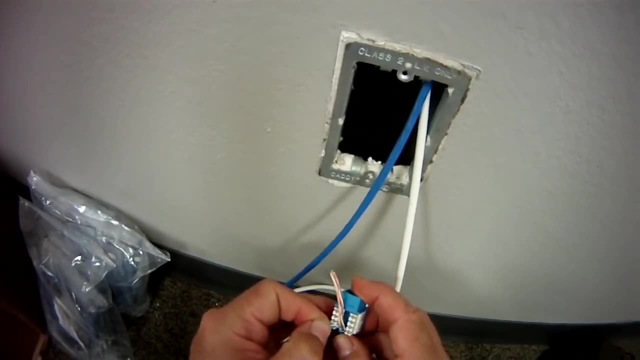 There's nothing wrong with A or B, at least in my mind. but I just do B, And what matters is that if you do B on your jacks, is that when you do your patch panel, your patch panel also needs to be done in B style. 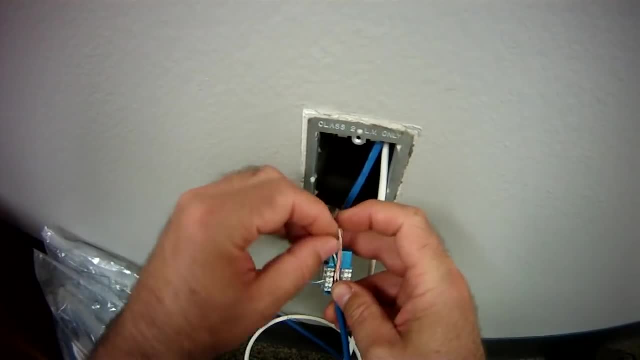 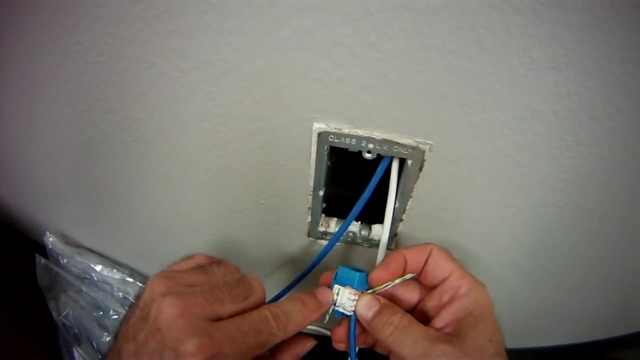 So that's what I'm going to do. Okay, so what I'm doing right now is I'm taking the wires and I'm spreading them out into the little grooves with the colors that correspond to the colors on the side of the jack. So I'm taking the orange pair here and I'm putting the white orange in. 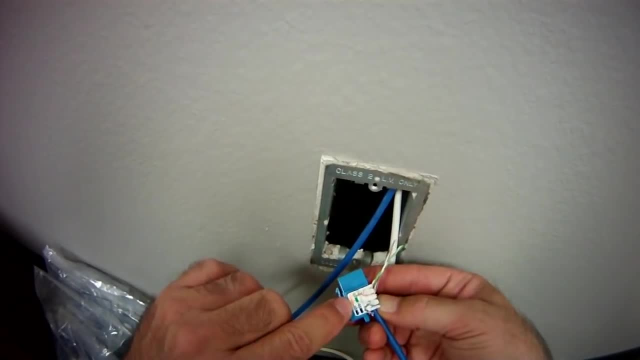 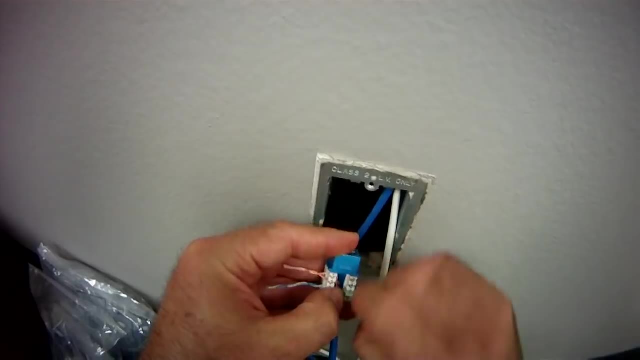 the front and the dark orange or the solid orange in the back corresponds to the pattern right there for B. And then, once I get that all done, I'm going to just double check it one more time, because an ounce of prevention is not going to. 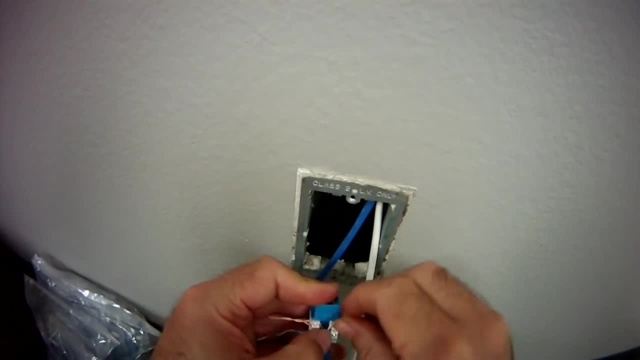 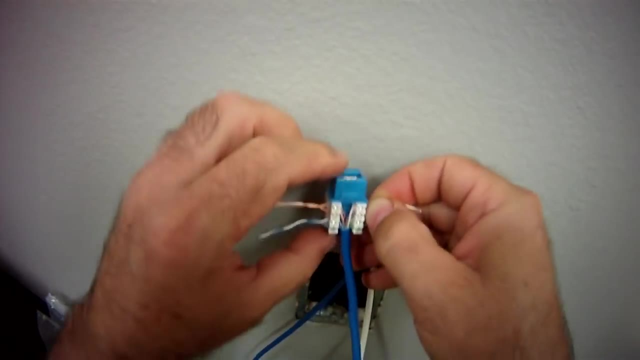 be enough. So I'm going to double check it one more time, because an ounce of prevention is certainly worth a pound of cure, because by the time you get this thing all put back together and then you go to test it, it doesn't work. it's. 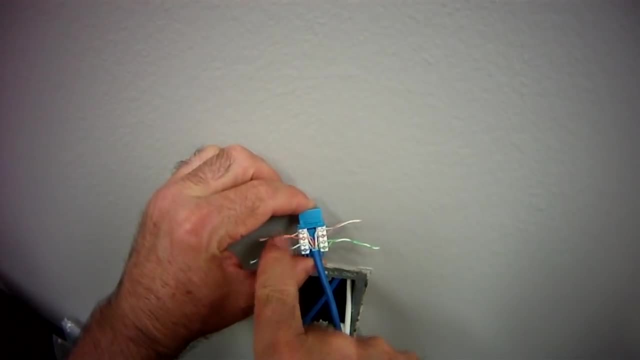 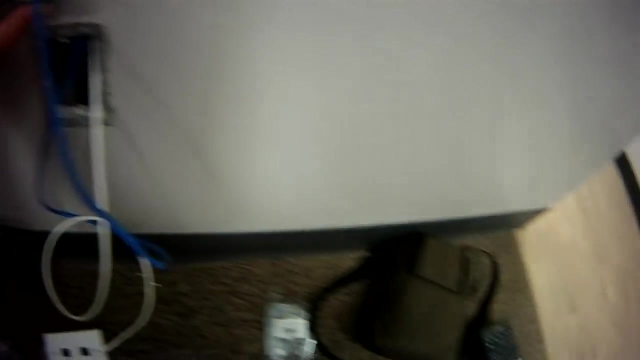 certainly worth having spent just an extra couple seconds to review your work. So what I do is I look and I say: okay, I got white, orange, orange, I got white, blue, blue, white, brown, brown, white, green and green. And once I've decided, 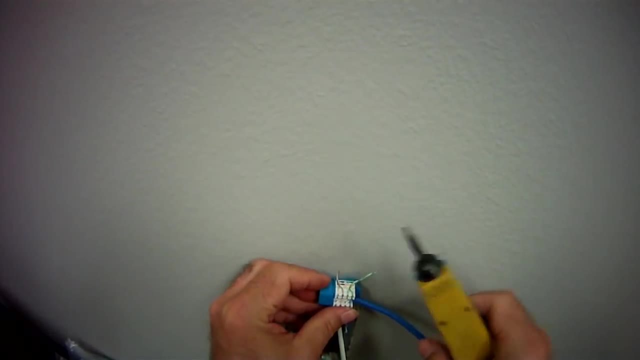 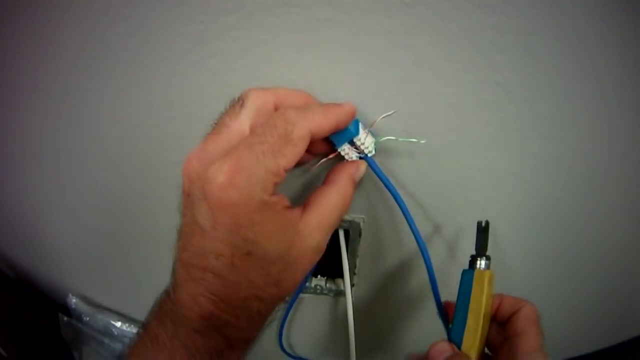 that. that checks out. okay, I take my punch down tool right here with my 110 and I'm going to go ahead and I'm going to terminate the jack. Now, when you do this, when you do it against the wall, it will scar the wall. So what I try to do is do it. 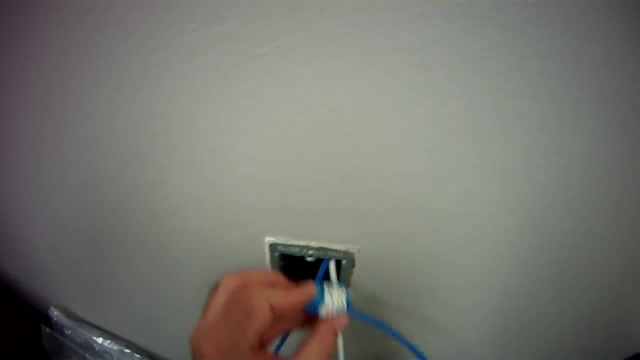 down near the outlet surface itself, because once I put the plate on, it'll cover up anything that it might have scarred by me doing this. As you do this, if you're doing it right, what should happen is the sharp end of the tool should be perforating or even breaking. 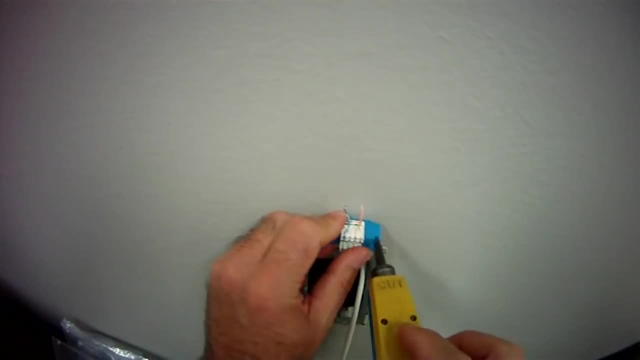 off the wire right there. Now you know…. Yeah, threw the excess wires into the wall and somebody called me out on that the other day, when i was making a video of a similar topic, and somebody said: well, why did you throw them in there? why? 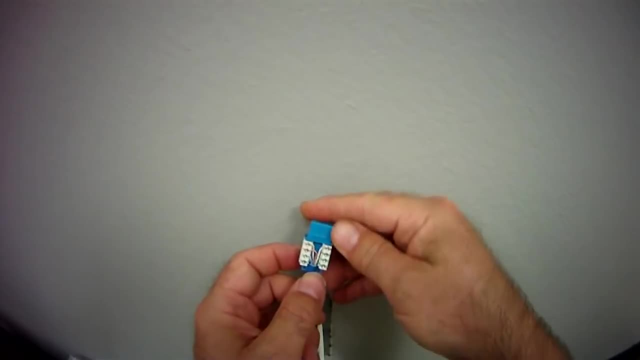 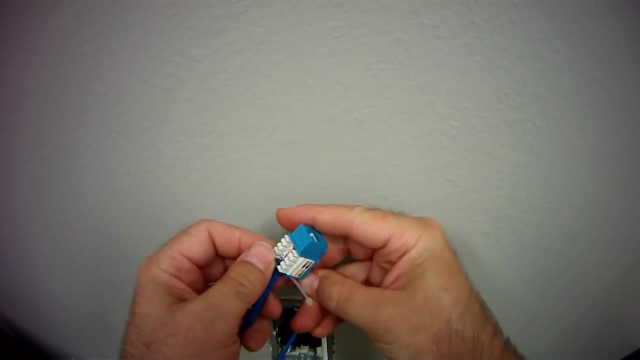 just go through my trash can listen for any of you trolls out there thinking about making comments about that. if you did this stuff day in and day out like i do, you would get tired of making trips to the trash. can, okay, throw a few pieces of excess wire inside the drywall, isn't? 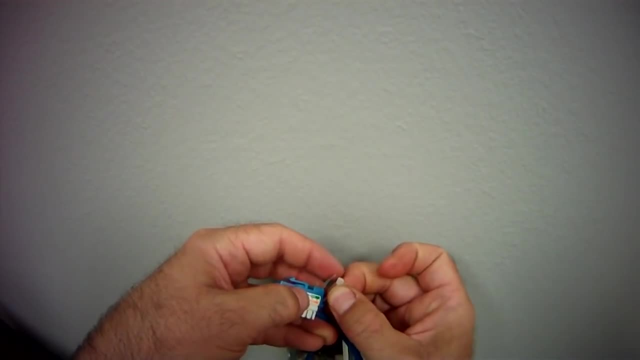 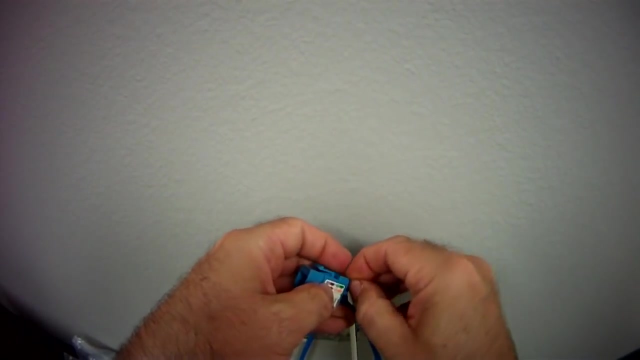 going to hurt anything. okay, now i also take this particular jack. not all jacks, but this jack comes with a little um piece of uh zip tie or a wire tie that you can wrap around the very base, which kind of helps reinforce the wire jacket right there. and if you do this, ideally the wire jacket 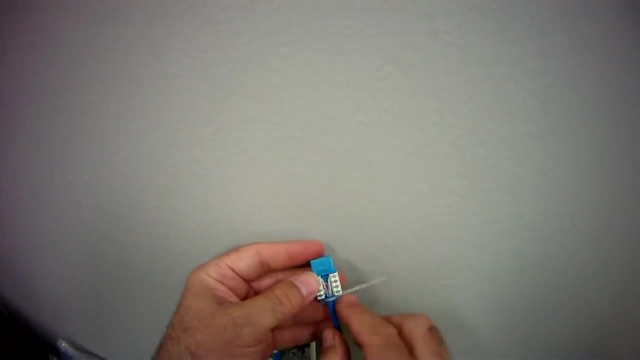 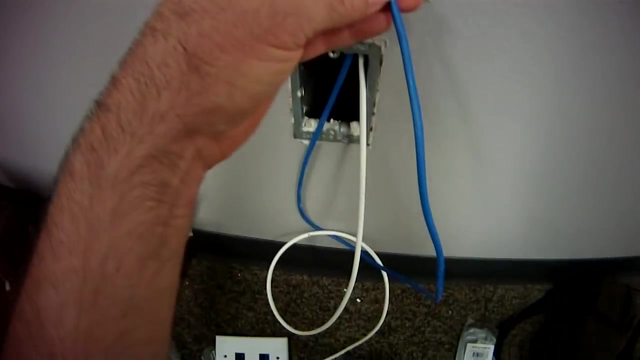 should mate right up against the bottom of the jack. where's the wire jacket. you shouldn't have a lot of exposed wire hanging out of the back of the jack. this one also comes with caps. most do come with caps, some don't, but most come with caps that you put on after you're. 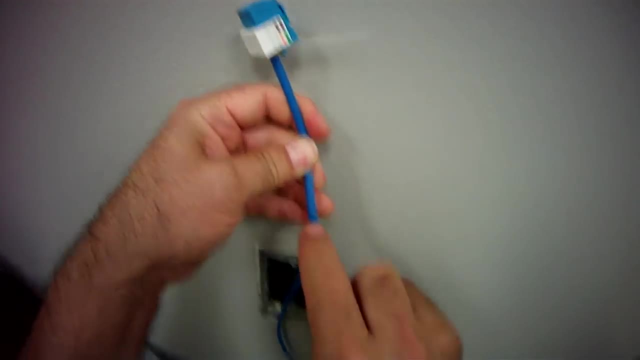 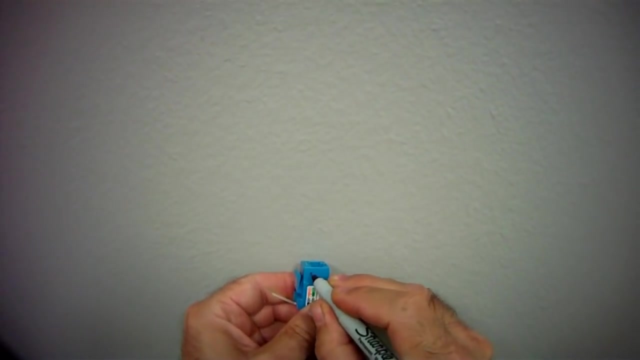 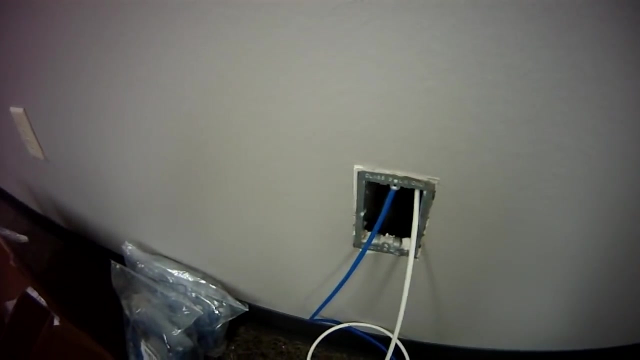 done also. what i'll do is i'll take- i wrote the number on the cable when i was pulling these earlier- is i'll take the number and i'll write it on the side of the jack just to help reinforce with a visual. that's my number. okay, then i'll also be. 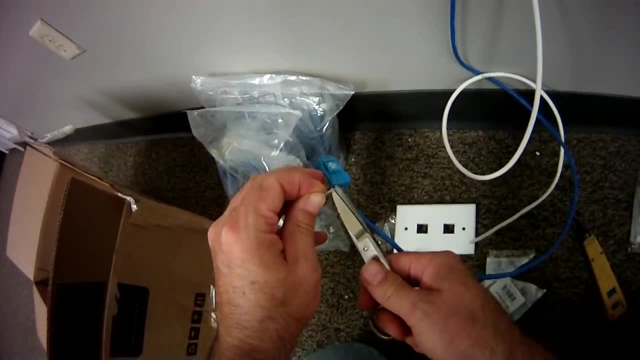 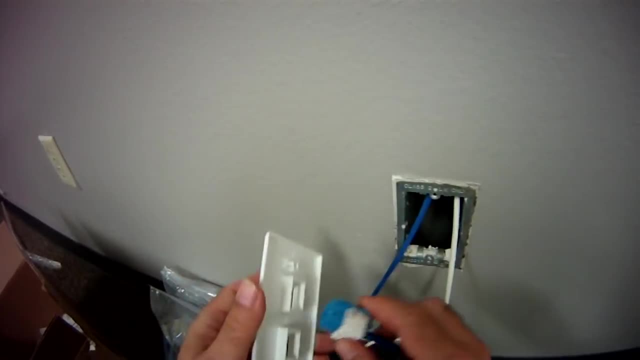 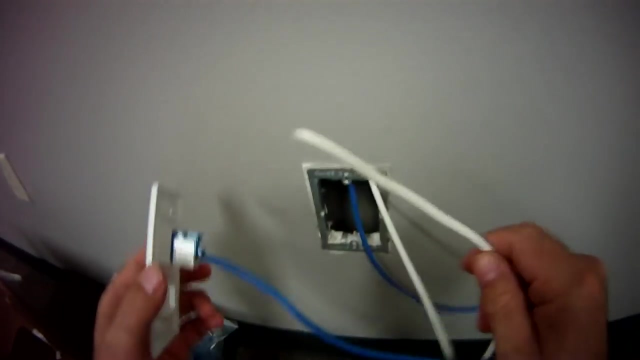 be a a. I'll be using a label maker to put um. i'll be using a label maker to put a three across the d3, across the top here. so i'm going to snap that into the back of the plate. okay, i'm going to terminate the white one now, and then, when i'm all done, that'll go in here too. i'll put the labels on. 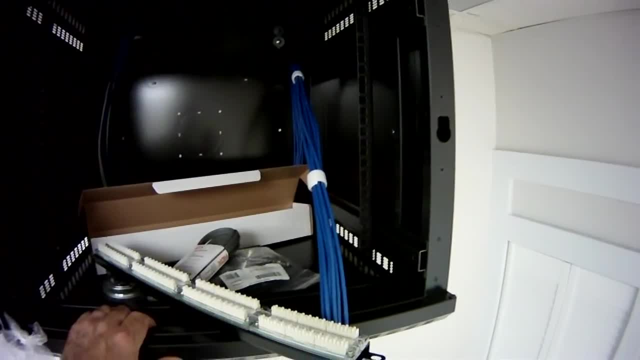 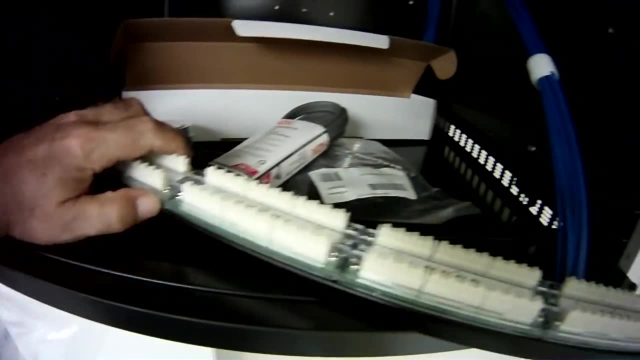 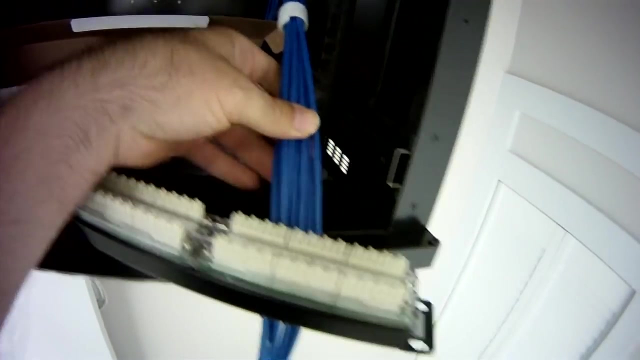 and put that into the wall. okay, all right. so now we've reached a point where i put all the outlets on all over the office and now it's time to terminate the patch panel. so, remember, this is my cabinet, where all the wires come to, all right. and here's all my my data cables and what i did when i was installing them. 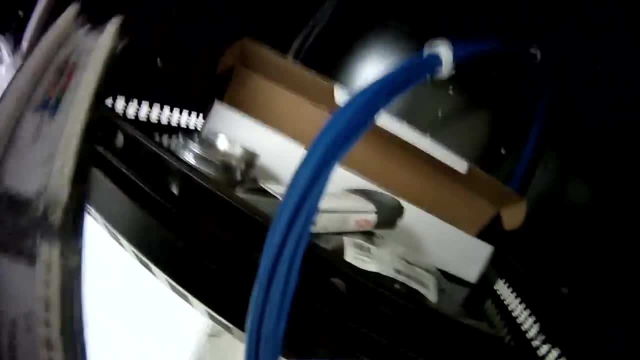 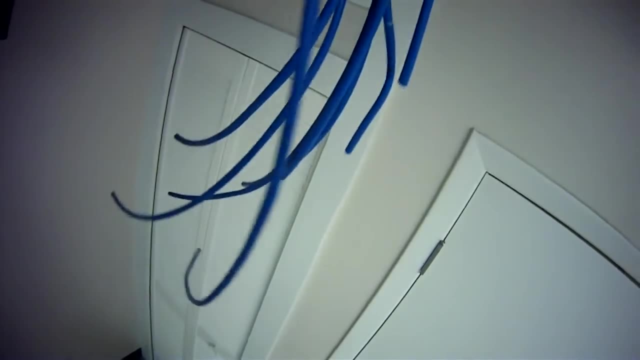 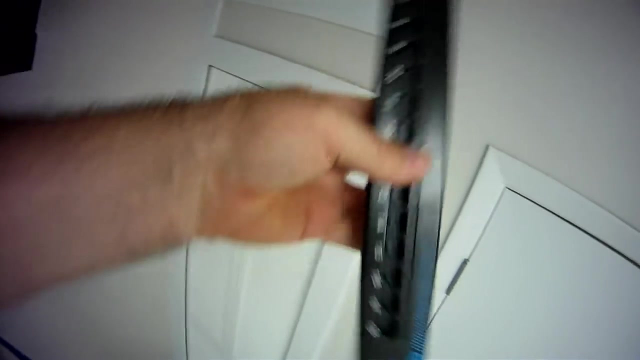 is. i wrote: whoops, i'm gonna drop something there. when i was installing the cables, i wrote the numbers on the end with the marker pen. so what i'm going to do is just like those jacks. i showed you that i was terminating. well, the patch. 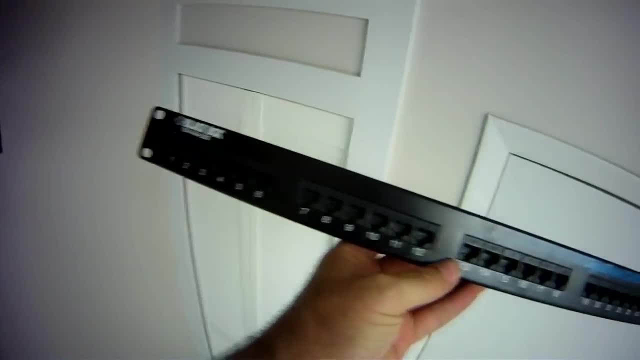 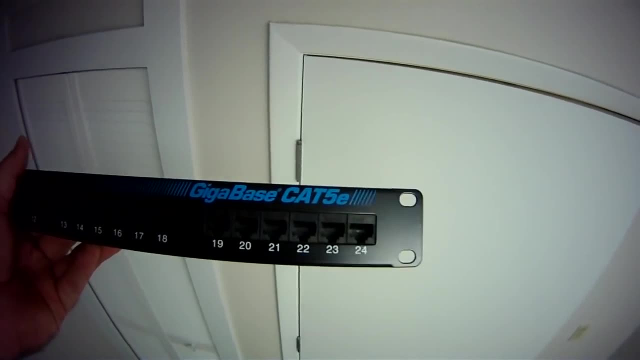 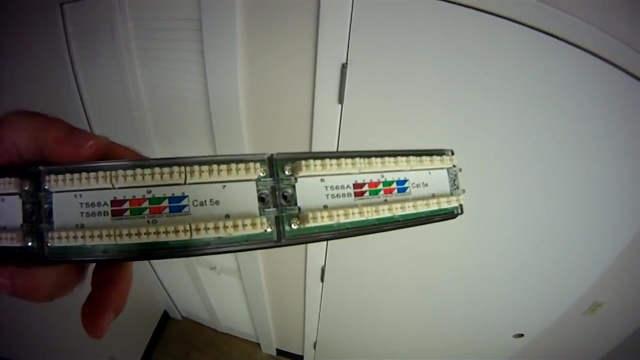 panel is just kind of like a like, a little bit more. like a little bit more, like a little bit more, a more aggregated version of the jack. So here I've got 24 Cat5 AP8C connectors. So on the back I've got 24 corresponding places to punch down the cables, And they're numbered 1,, 2,, 3,, 4,. 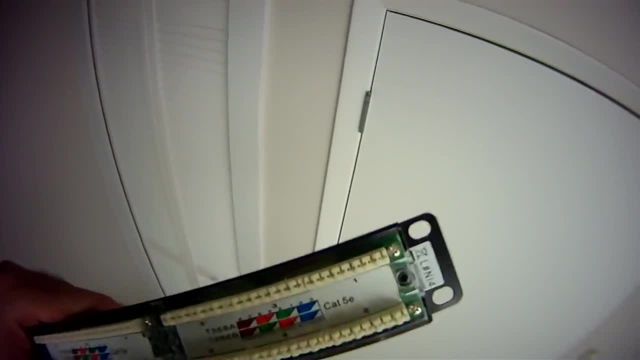 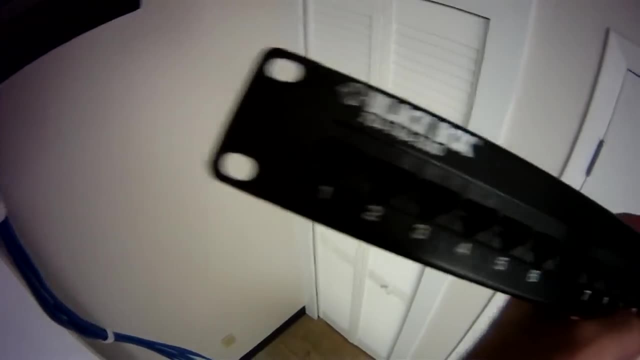 etc. So what I'm going to do is take my cables in the number that they're ordered and match them up with the numbers here and punch them all down, And then I'll have a complete network pathway between the numbers here on the front and the jacks out there with the corresponding numbers. 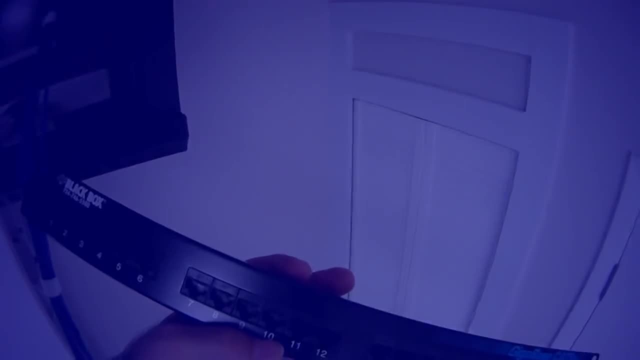 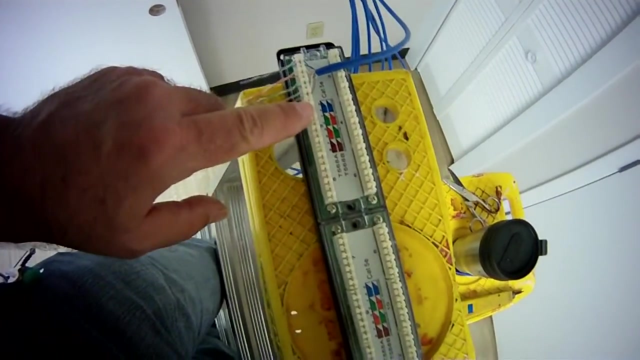 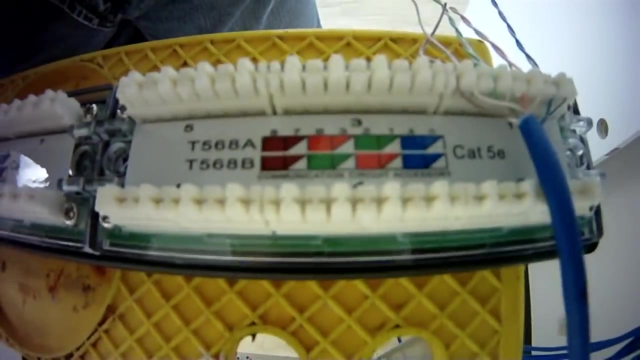 So let's get that done. I'll show you what that looks like. Terminating the patch panels is really no different than terminating the individual jacks, except now all the places for the punch downs are all just very tightly integrated together. As you can see, there's the same pattern there. The top one is 568A, the bottom one is 568B. 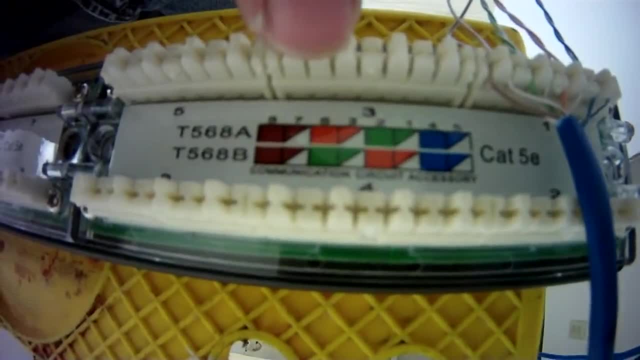 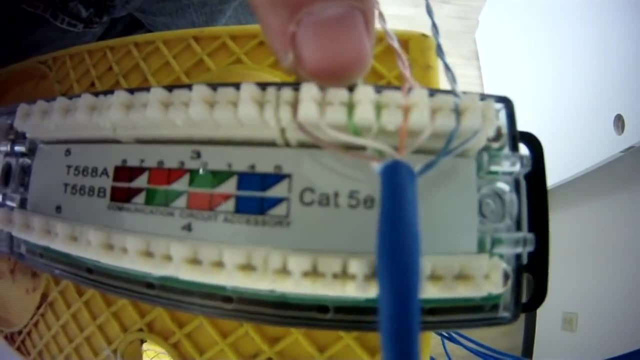 So see how it's got, like a white-blue, then solid blue, white-orange, solid orange, etc. And this is under the B section. So that's what I did. I've got white-blue and blue, white-orange and orange, white-green and green, white-brown and brown. 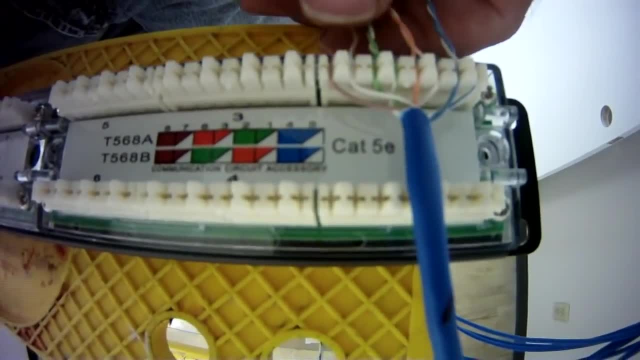 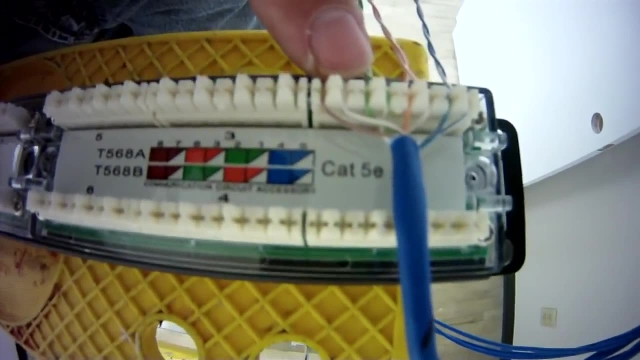 And so there's a couple of different ways you can do this. Some people prefer to lay out all their stuff first and then do the terminations. I kind of like to go one or two at a time, So I'll spread one out like that, in kind of that Y shape. you know where the orange and the green. 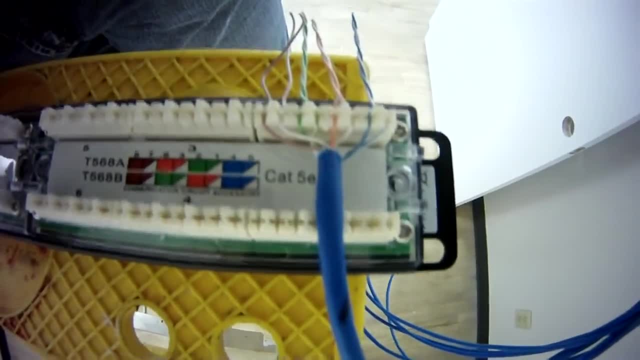 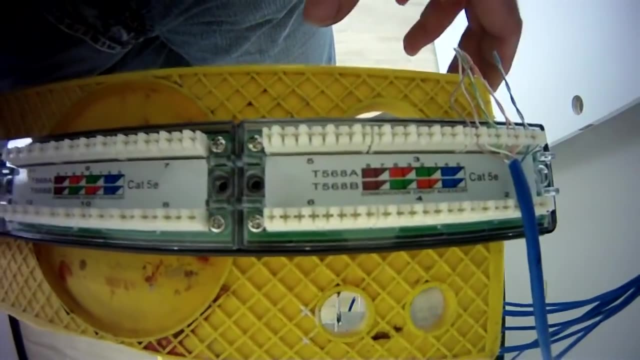 are shorter, and the blue and the browns have to stretch a little more to reach the outsides, And then I'll go ahead and terminate those, And then I'll go on and do number two, and then three, and then four and five and six, etc. And so on. So this is nice to do when you're doing a brand. 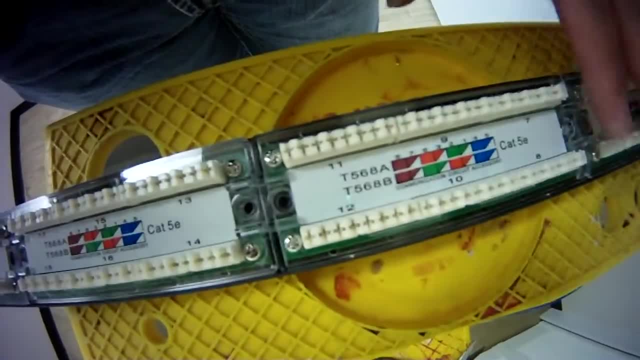 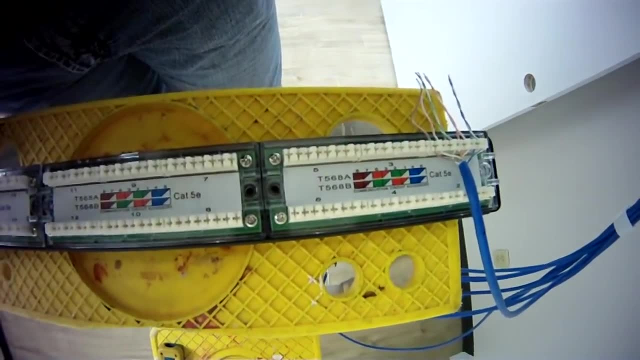 new installation, because you can actually take the patch panel and lay it down on something flat like this and terminate the wires. Unfortunately, when you're adding a wire to a system that's already been installed, you kind of have to, you know, reach up inside the cabinet and terminate. 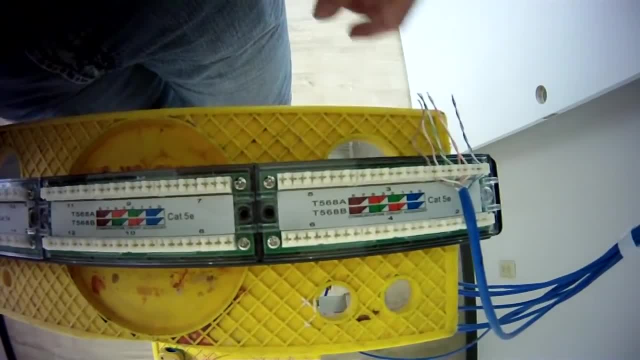 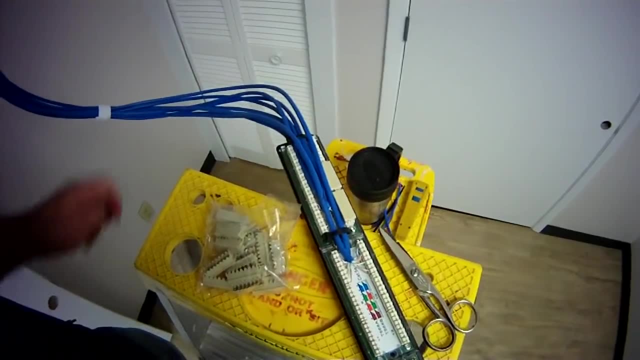 the wire on the back of the patch panel while it's already mounted. So I'm going to get that done and show you what that looks like when I'm all done. Okay, now the patch panel has got all the eight wires Terminated on it, And this one comes with these little caps that you can put on the back. 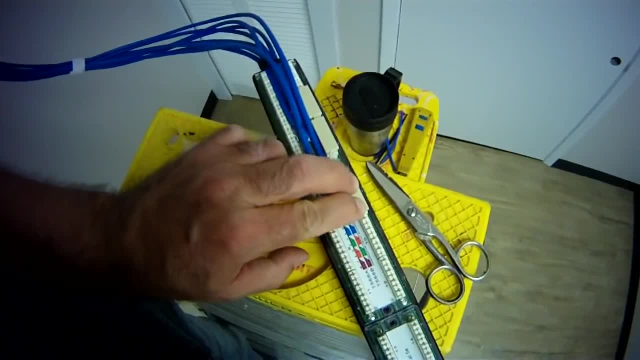 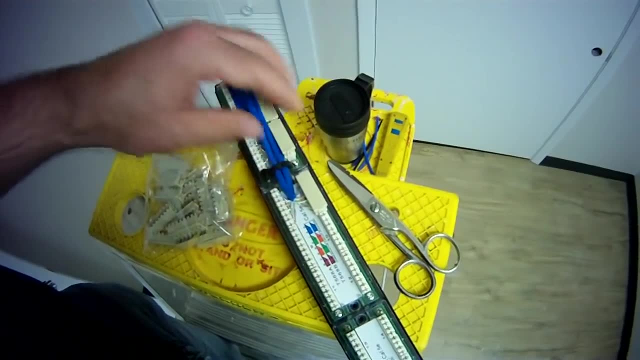 They kind of help- oh, I guess you know block off air and maybe you know, help reinforce the connection. I personally am not a big fan of those because I believe that if you do your wire management right and you've done your terminations right, there's no reason why those wires should. 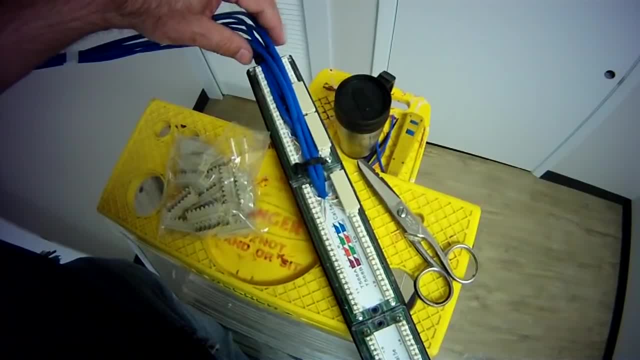 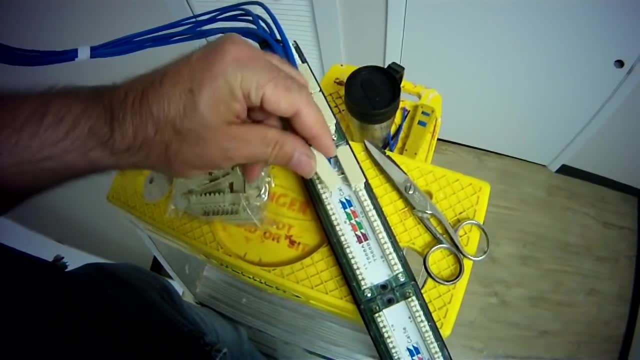 pop back out of there. They'll come out of there if your wires are not managed correctly and there's too much tension on them, pulling them out of the sockets. But anyway. so if yours comes with the caps, you can go ahead and put the caps on, It doesn't hurt. 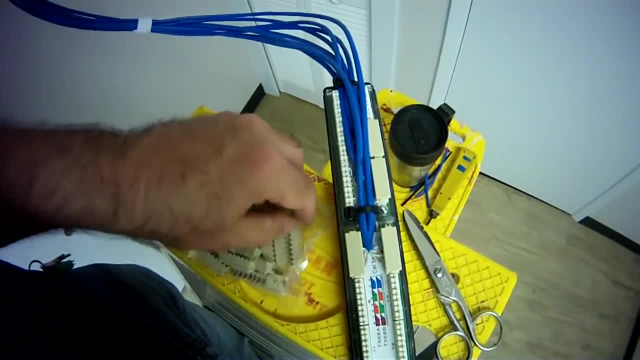 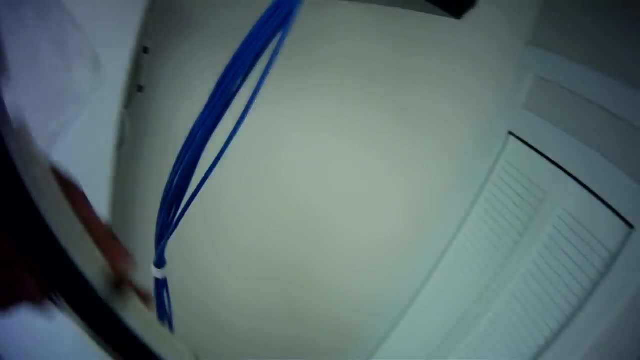 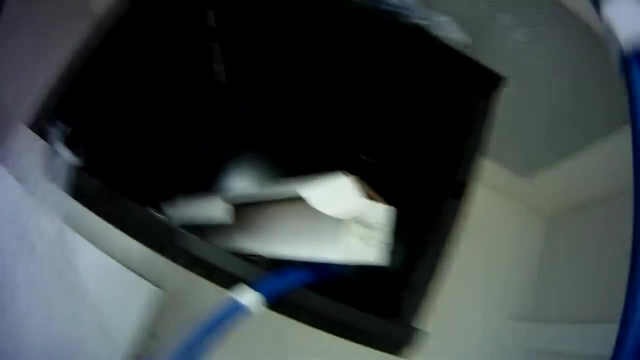 anything Like I said. I'm just not a big fan of the caps, Anyway. so now that my terminations are done, what will happen next is I'm going to have to re-manage my wire back into the cabinet, So basically taking this slack and just kind of dressing it in there along the walls And then 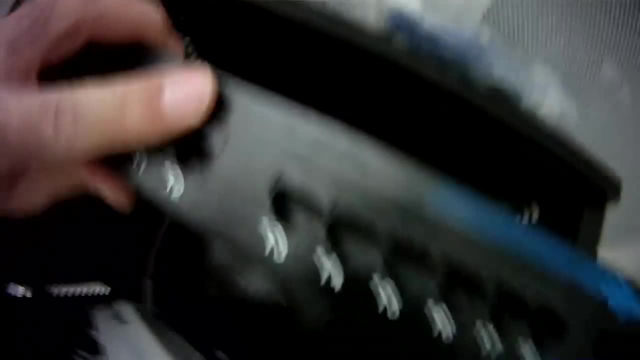 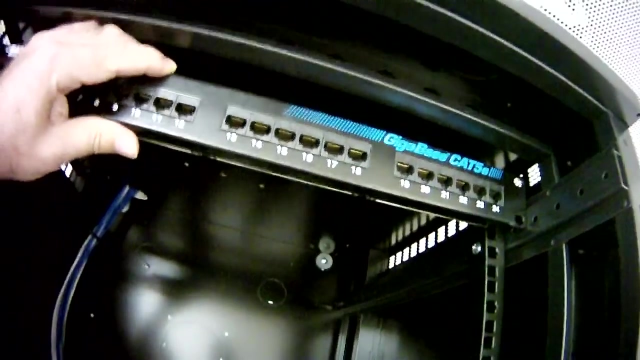 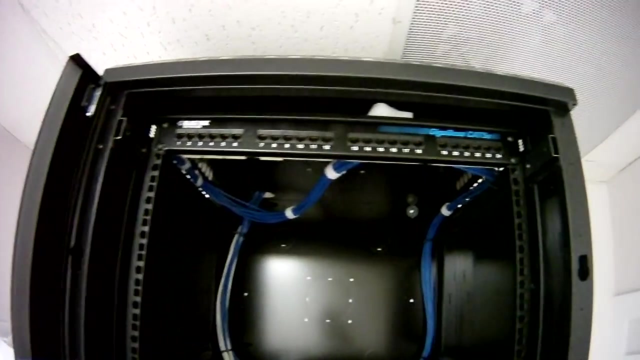 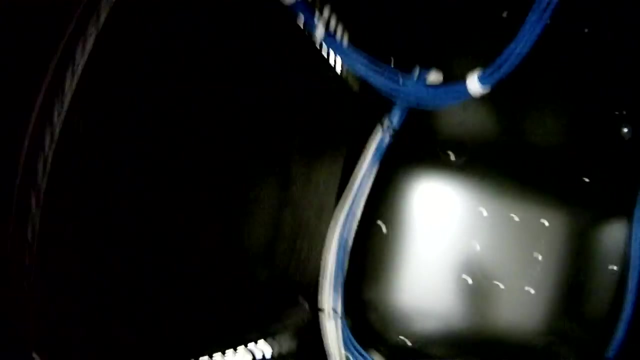 ultimately, my panel is going to get mounted Up in there And then I can start doing testing on my outlets and my patch panel. Okay, I'll show you that in a little bit. All right, so the patch panel is done and mounted And you'll notice that there's this maze of the 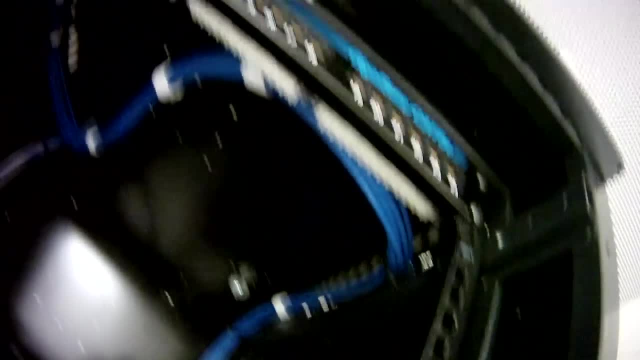 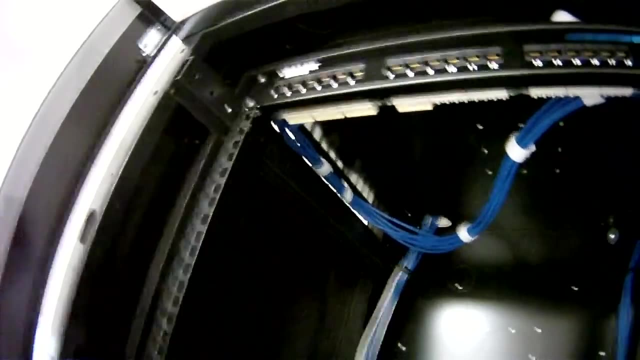 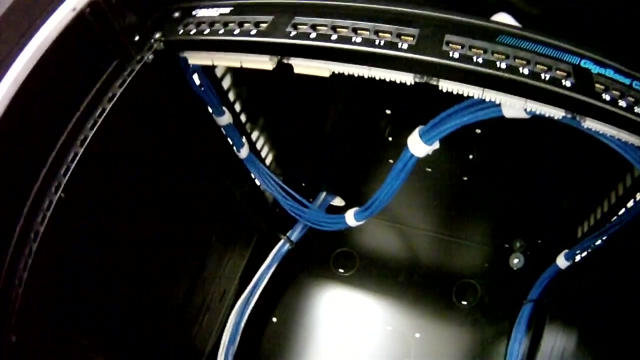 wire running around and down and up and across. That's actually for a reason, And I may have gone a little crazy with that, but that's known as a service loop And it's there for a couple of reasons. One is if for some reason, something happens to the cable near the patch panel. 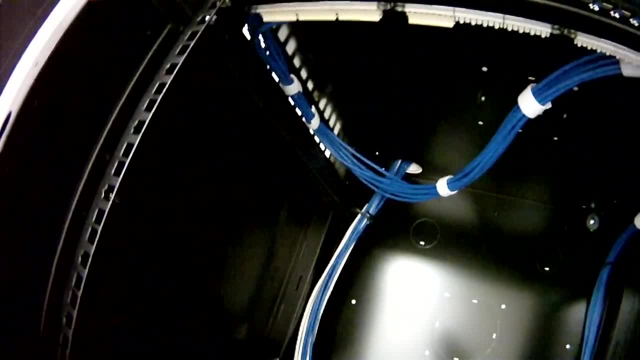 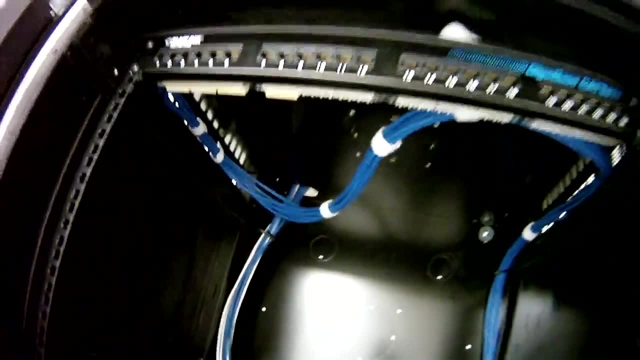 it gives you the reserve amount of slack to be able to pull some more slack and re-terminate the cable And it's cut off the end and re-terminate it. The second thing it does is it gives you the flexibility to move the patch panel. So say, the network configuration changed one day and we need 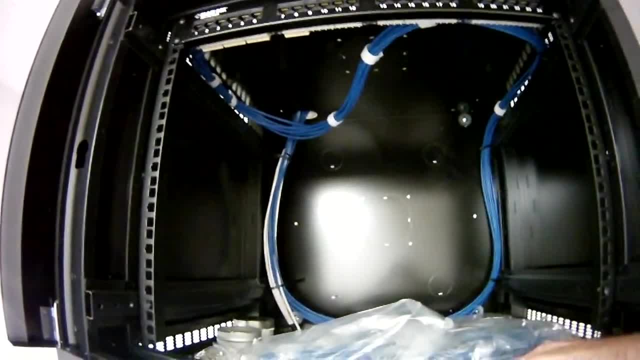 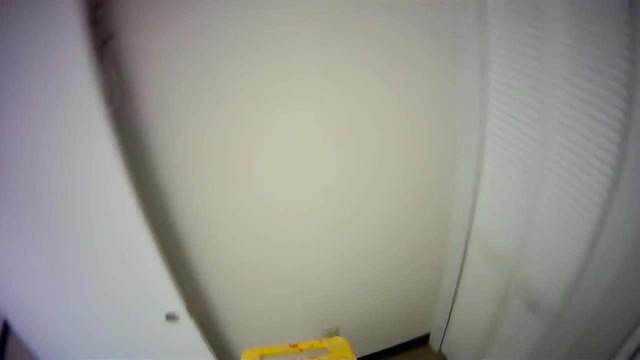 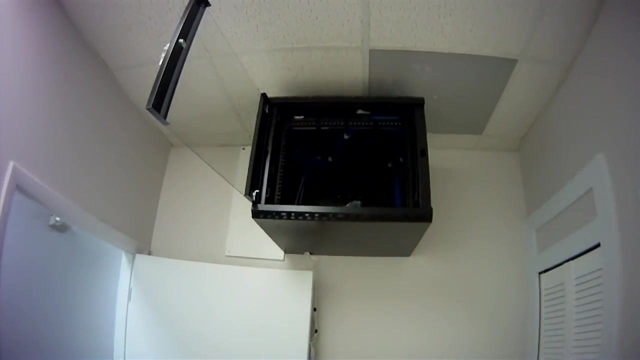 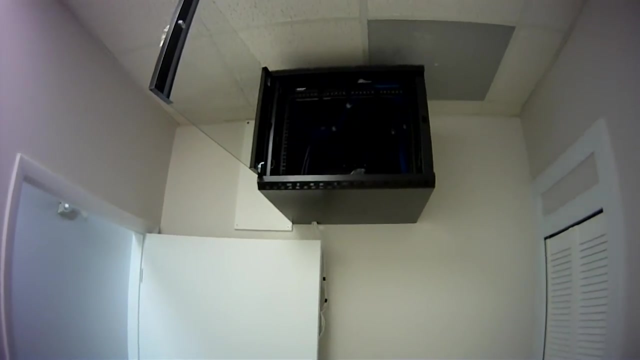 put in like a floor-mounted network rack, say over here in this corner by the closet. I've got a good six feet of slack that I could move that patch panel without having to re-run all those cables again. And also, while we're on the topic of the network cabinet, this just happens to be the one- 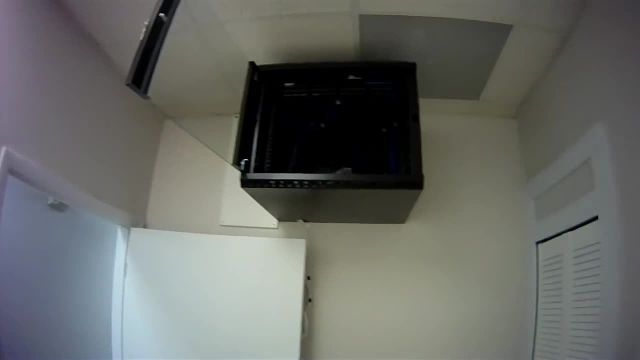 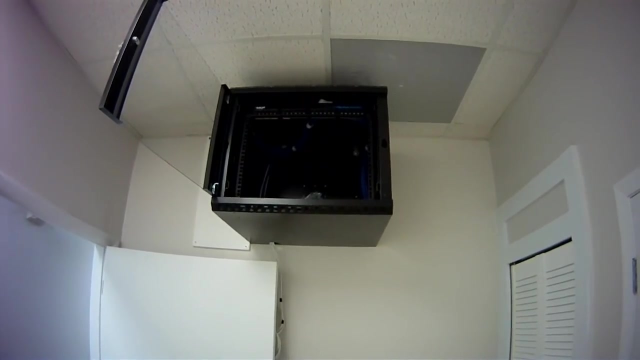 that I'm using for this doctor's office. You don't need to go get one of these big network cabinets. You can simply get a patch panel and a one-u or two-u hinged brackets that you just mount on the wall. So all you would really need. 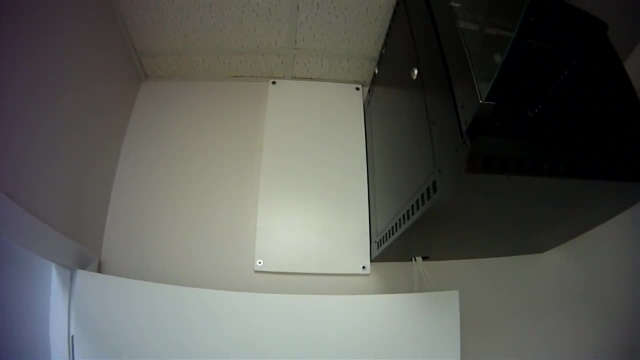 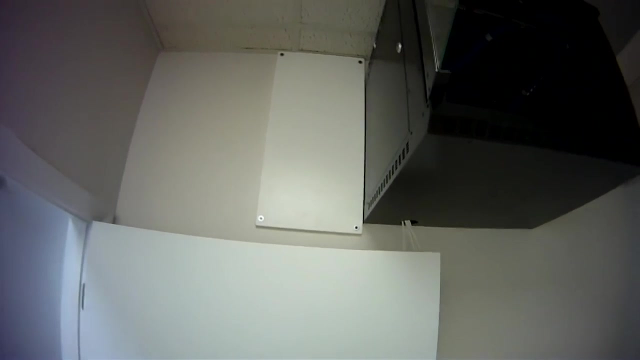 for instance, is like this little white board. You could just get a little white board like that, mount it horizontally instead of vertically, and then you could put the little hinged bracket on there with a patch panel. Okay, those are very inexpensive. The hinge brackets, I think, are. 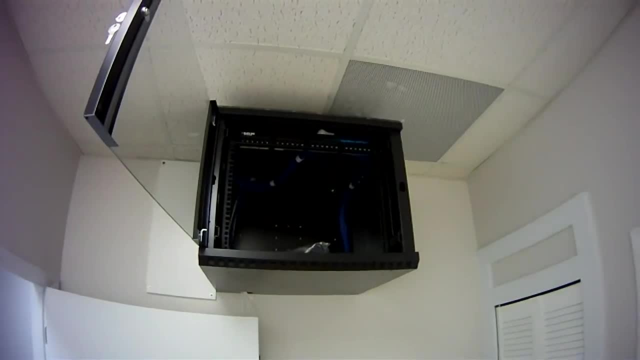 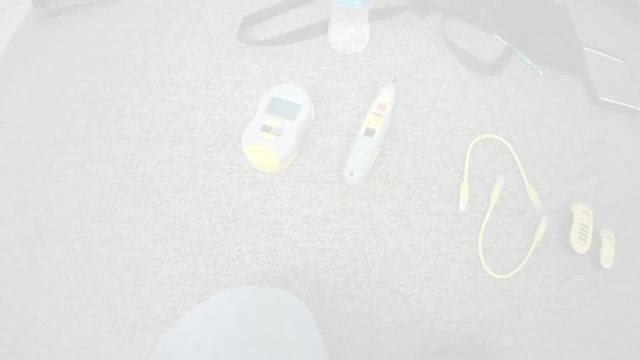 about 20 bucks. You could get inexpensive patch panel off of Amazon or a mono price for probably about the same, about $20.. Okay, now I'm going to go ahead and move this panel down to here. I'm going to begin the testing. Okay, so now I'm down to testing. So I've got two different ways. I 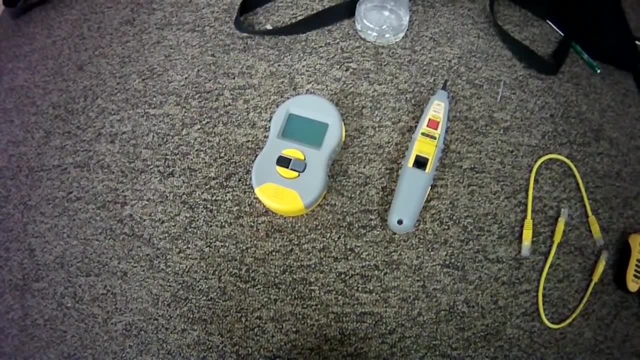 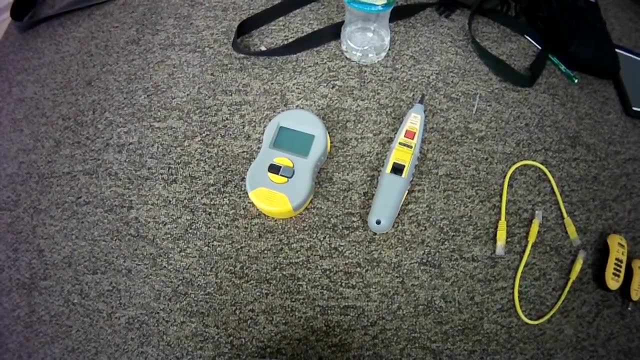 can test. This thing you're looking at right here is called a certifier. It's an expensive piece of equipment that's designed to stress the wire and test it for its maximum capacity, to certify that it's either Cat5 or Cat5e or Cat6, etc. I recommend, on the other hand, that you use something simple. 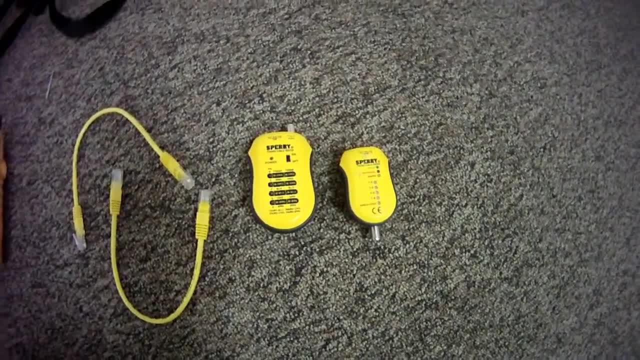 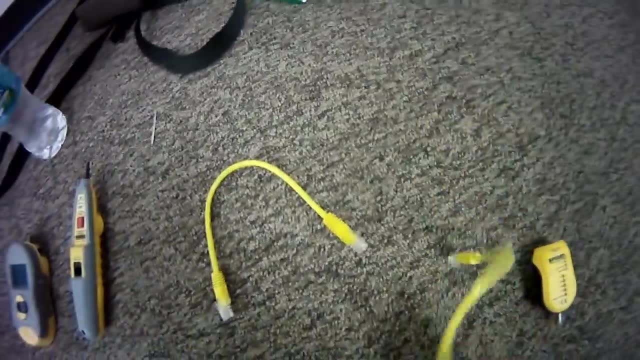 like this. This is just a continuity tester and it works really simply. It's got an RJ45 or an 8P8C on both ends and when it's connected to two ends of a cable, it simply sends current down the line. 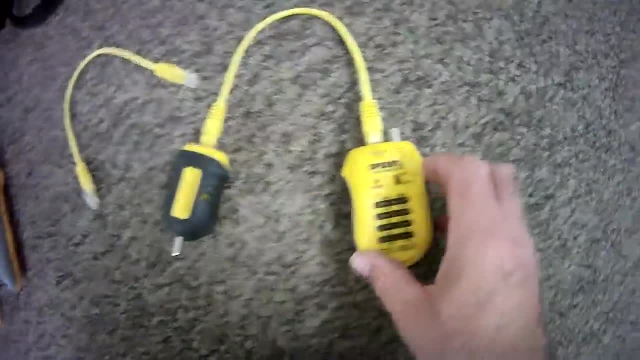 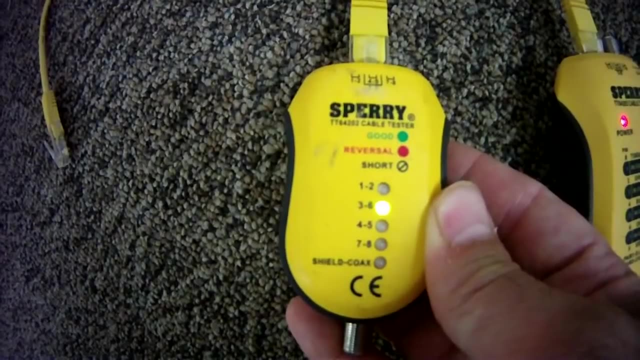 on each pair. Okay, so I'm going to turn it on right now, and what it does is: at the far end you should see these little lights turn green in order. If any of them are red, or if it goes out of order, or if one of the lights doesn't light up, that means there's something wrong with either. 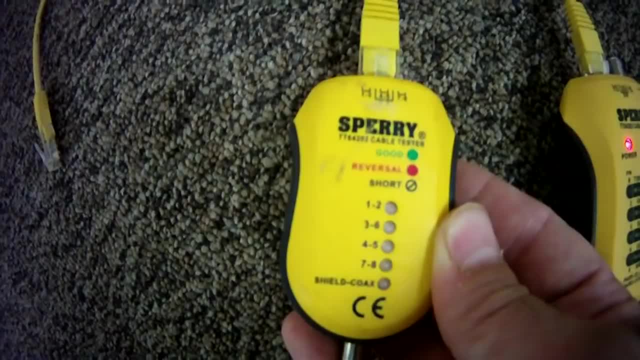 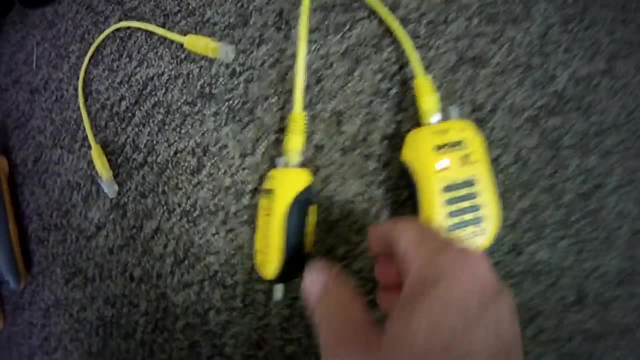 the cable, but most likely what's wrong is it's something that you terminated incorrectly. So either one of the ends of the jack is either not terminated right or didn't get terminated all the way Okay. so again, I'm recommending you just get a continuity checker. I have to use this special. 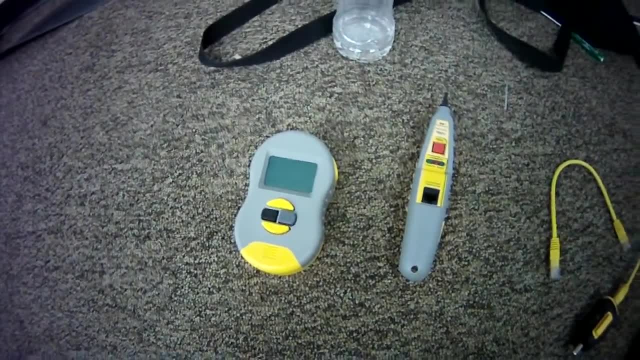 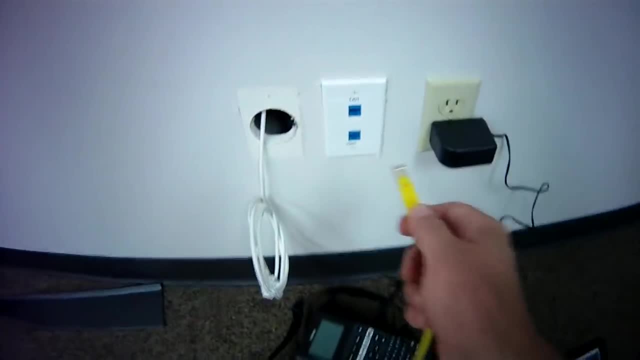 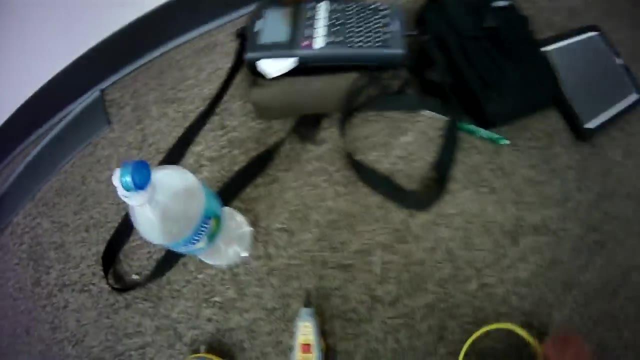 certifier tester, because I'm doing work commercially and I have to provide results to my client. All right, so let's show you how this works. So let's take, for instance, D1.. So plug my little continuity tester in D1.. I've got it turned on. Then I'm going to take this other little guy.